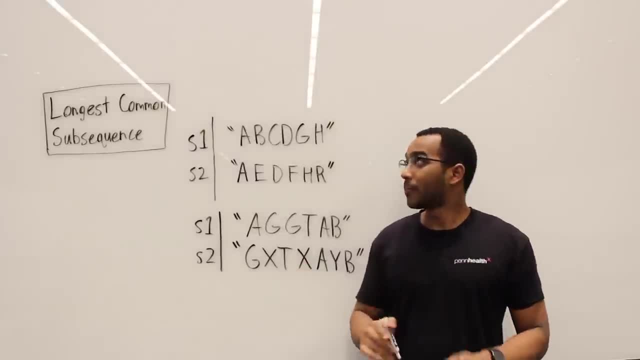 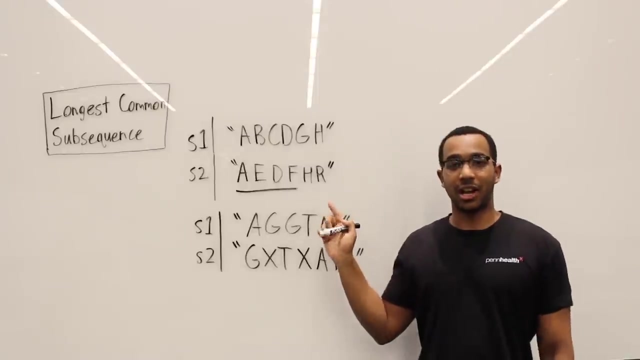 approach for this. Okay, so how does this problem work? So we're looking for the longest common subsequence. When you see, subsequence that means that what we are looking for does not have to be contiguous. What does contiguous look like? What I just underlined is a contiguous sequence, That is. 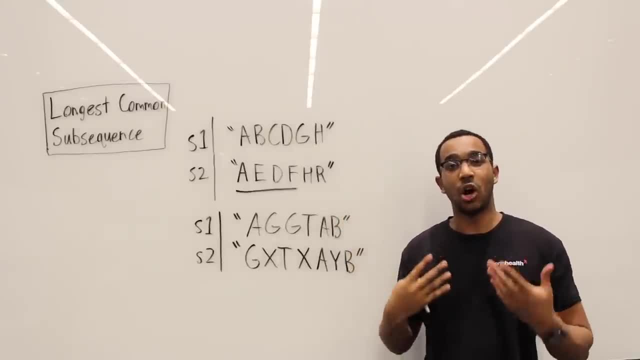 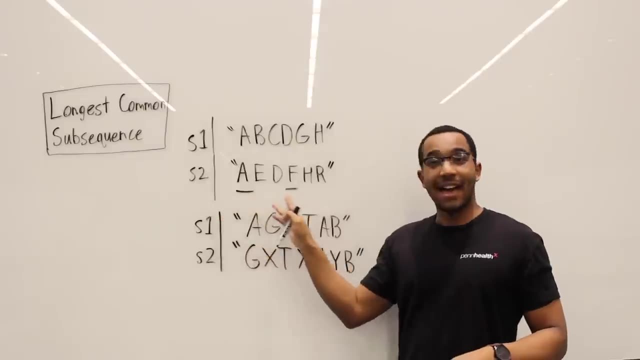 all together. There's no gaps. What can I do to make it non-contiguous? That sequence- right there- is not contiguous, So this is a subsequence. AF is a subsequence. A subsequence does not have to be contiguous, But it can be contiguous. A subsequence can be contiguous. It might be broken up like this: 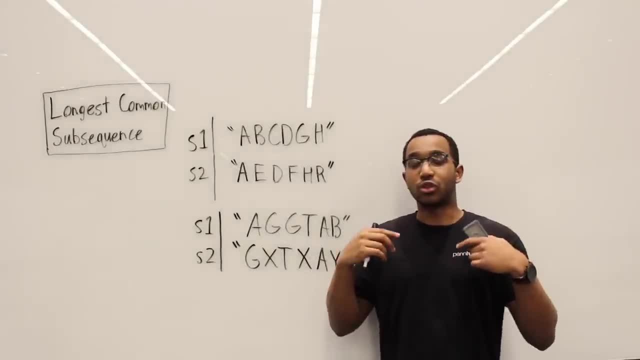 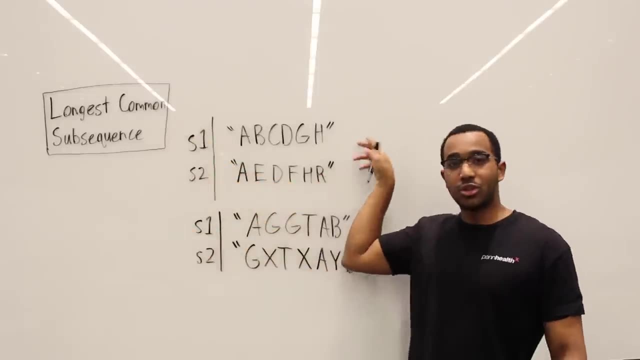 It could be both of them, All right. so our job here is to return to our caller the length of the longest common subsequence between two strings. So what is the longest common subsequence here? So we see that they share A's, and we also see that these strings share D's, and we also see: 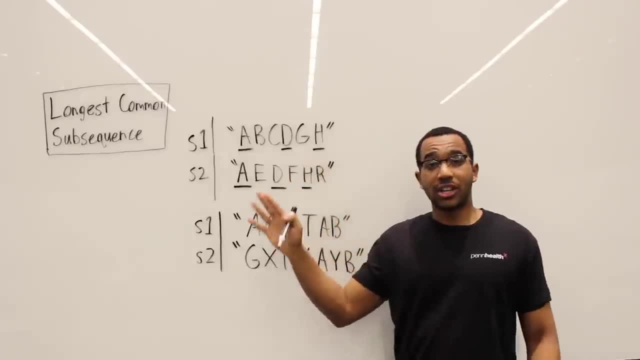 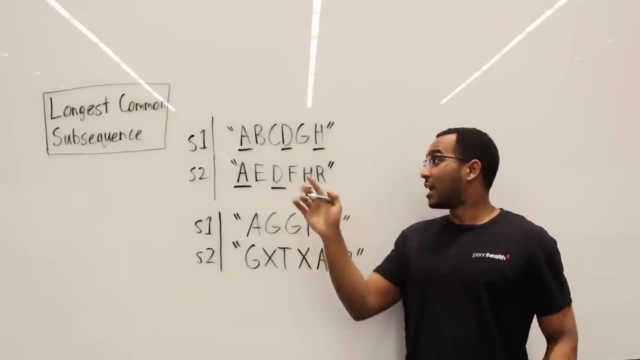 that these strings share H's. So the longest common subsequence here is the longest common subsequence between two strings. The longest common subsequence, The longest subsequence that these strings have in common, is ADH, ADH. How long is that? Three? So what we return to our caller is three. So looking at this, 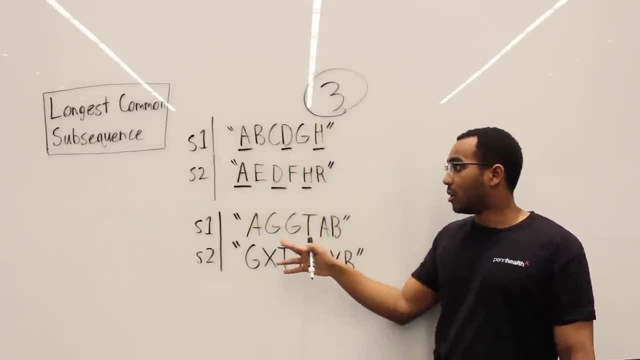 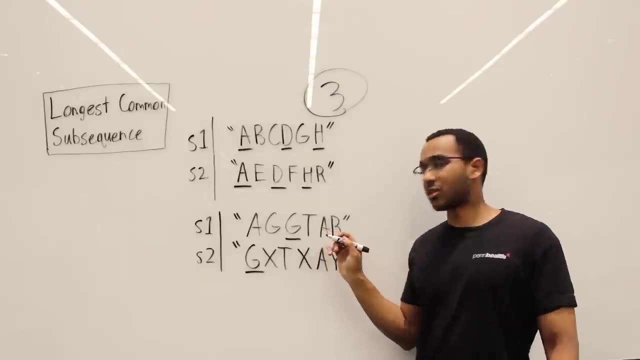 example, what is the longest common subsequence? So the longest common subsequence is: we see they share G's, but we're going to underline this G. We see that they share T's, We see that they share A's and we see that they share G's, So what we return to our caller is three. So, looking at this, 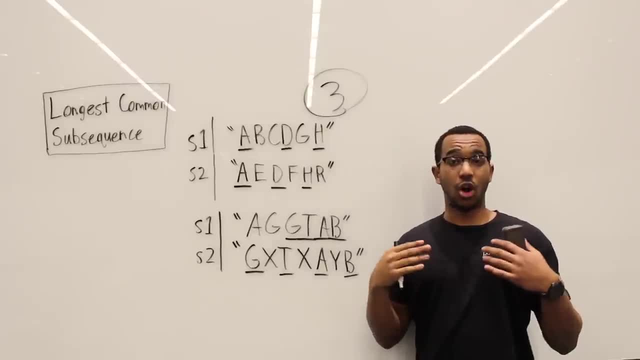 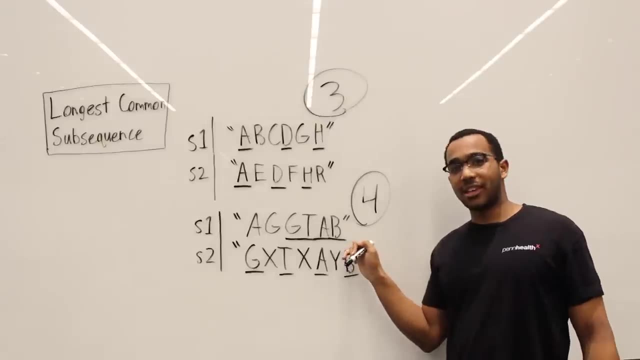 example, what is the longest common subsequence? So what is the longest common subsequence? We see that they share B's. So what is the length of the longest common subsequence for these two strings? It's going to be four. Okay, so you see here that this is contiguous. but again, this guy right here. 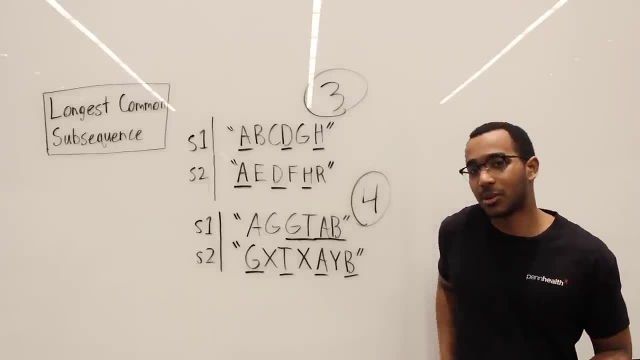 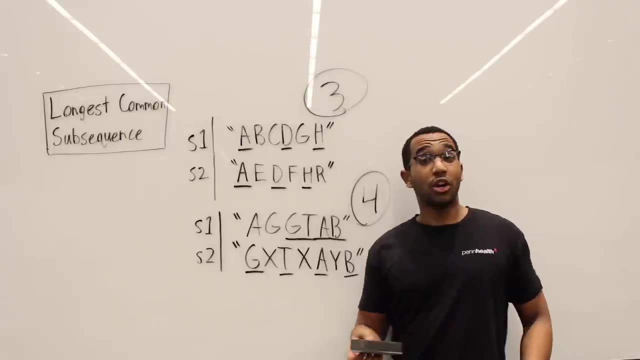 is not contiguous. These are subsequences. They don't have to be contiguous. So this is our job and, as I said, what we're going to use is dynamic programming for this problem. We could try to brute force this problem. We could try to generate all subsequences. This would be. 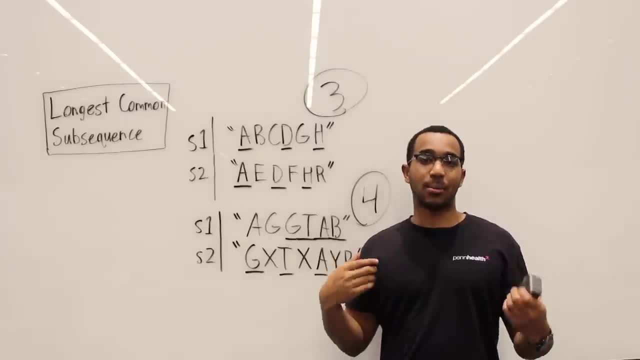 again exponential in time. So what we're going to do is we're going to use dynamic programming and I'll explain why or how we would get to this in an interview, because most of the time you probably wouldn't, and these are difficult problems to do, but we'll see how we can wrap. 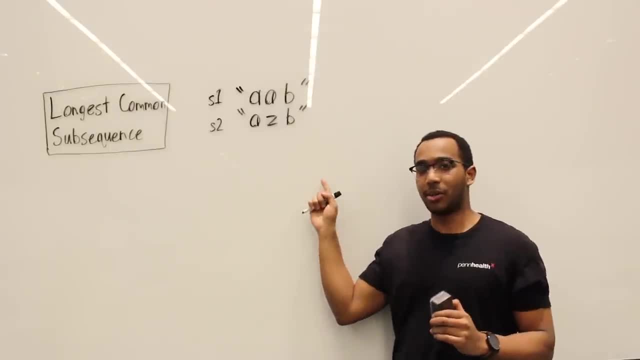 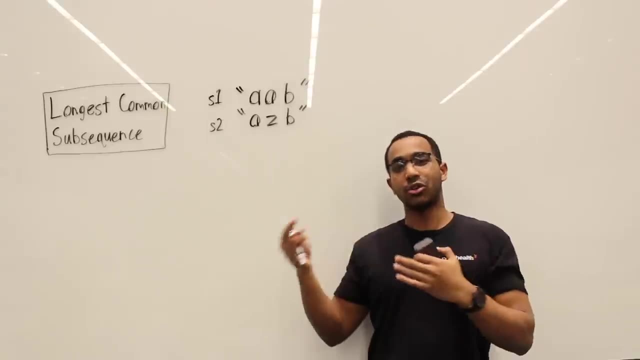 our mind around this question. So I created a little example here and I want to help you wrap your mind around this problem and gain a deep understanding of what we're going to do. later We'll get into our DP table, We'll do all of that stuff, but what am I really doing? What are the 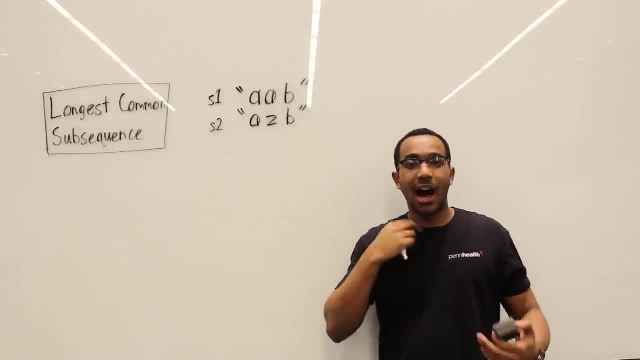 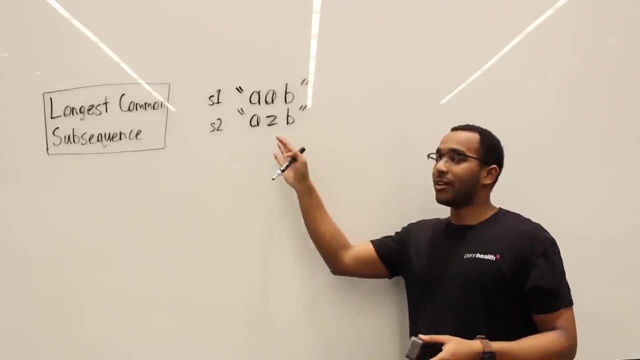 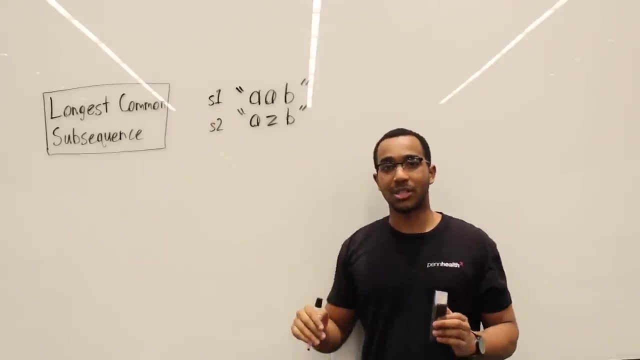 like subproblems. Whenever I do dynamic programming, I care about subproblems, remembering the answer to subproblems and things like that. So what we have here is two strings. So my job is my job is to find the longest common subsequence of these two strings. 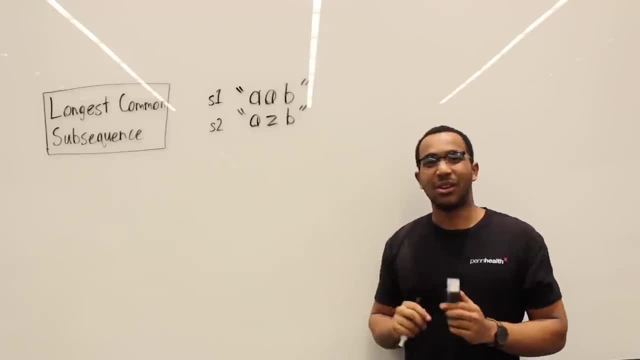 So what I'm going to do is I'm going to break this down into a call recursion tree. So what I'm going to do here is I'm going to break this down into what each common subsequence is and I'm going to break this down into a call recursion tree. 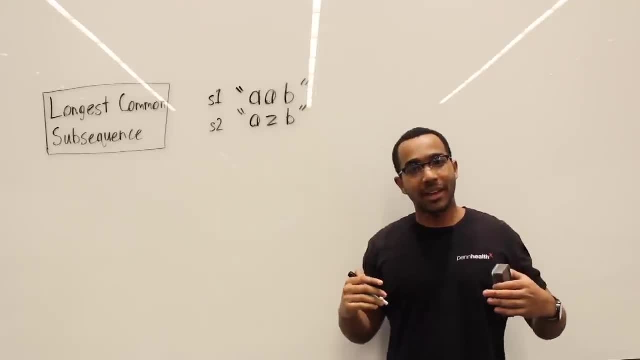 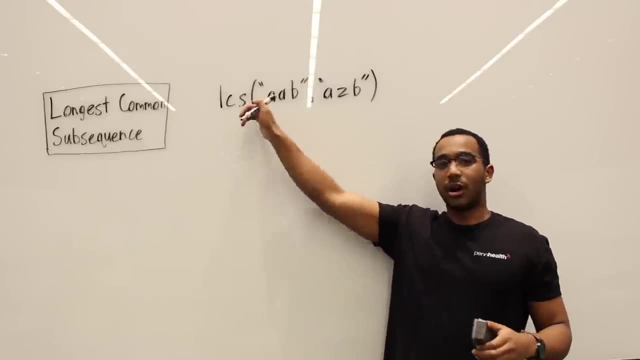 So we're going to see what each call looks like and what decisions we make at each point based on what we see. So stay with me, So watch what happens. Okay, so we have longest common subsequence called on these two strings. This is just pseudocode or like. this isn't even a real 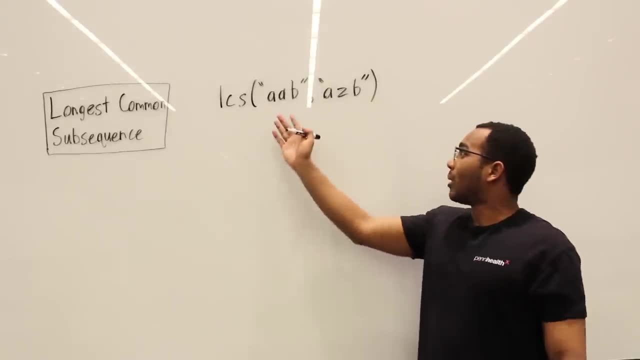 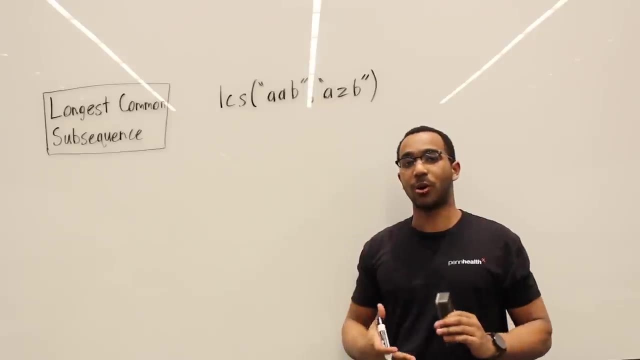 function. but let's just imagine this is our function. So what we have is string one and string two. So what I'm going to do is I cut this up into subproblems. This is the hardest part about solving dynamic programming problems. 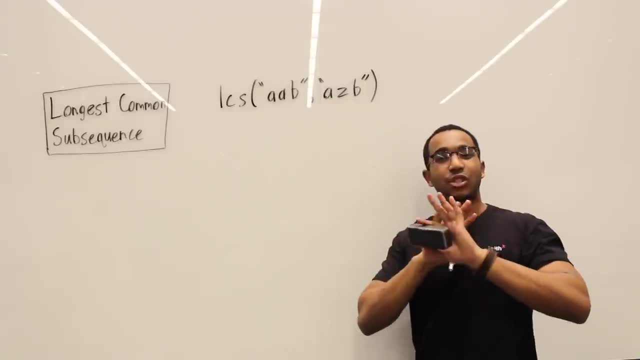 So I'm going to look at the last character. That is all I care about. Okay, I have my eyes on the last character And what do you see? Are these characters the same or are they different? So we see they're the same. So what does that mean? That means I have a lengthening of my longest. 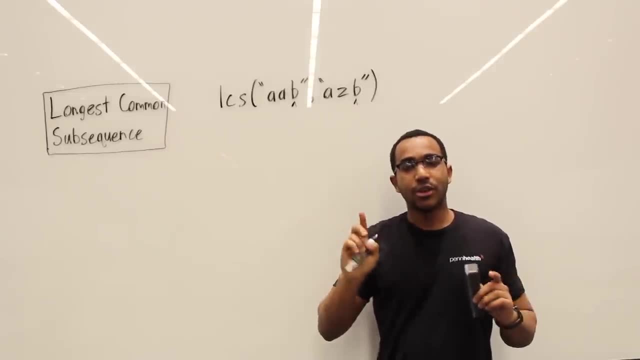 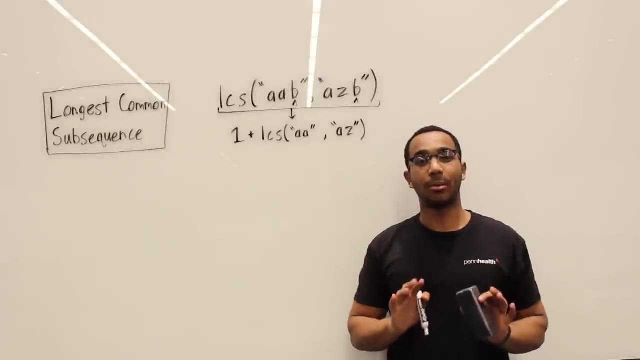 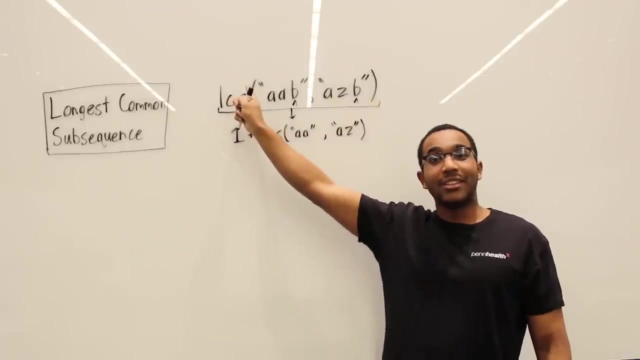 common subsequence by one value. So what happens is: this is what happens. So do you see what happened? I broke it down into sub problems. My eyes were on the last character And what I'm doing now is I said what's the answer to him? The answer to him is one plus the answer to this. 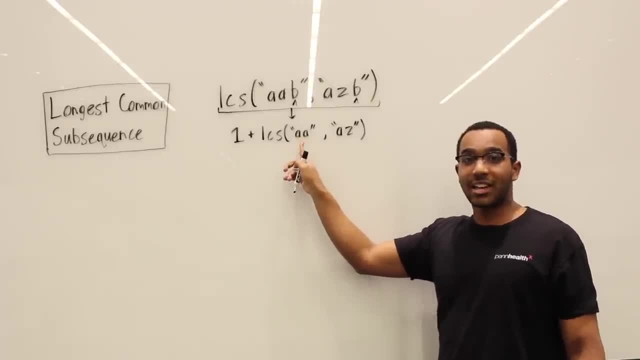 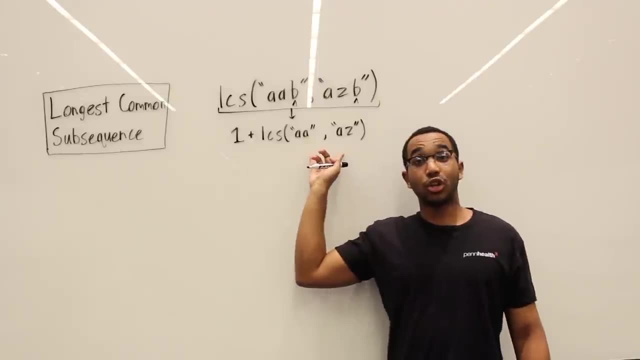 guy right here And you see, we broke it down. We cut off the last character, We cut off the last character. So the answer to this is: we chop off the bees. And now, what is the longest common subsequence problem? What is the answer to the sub problem? 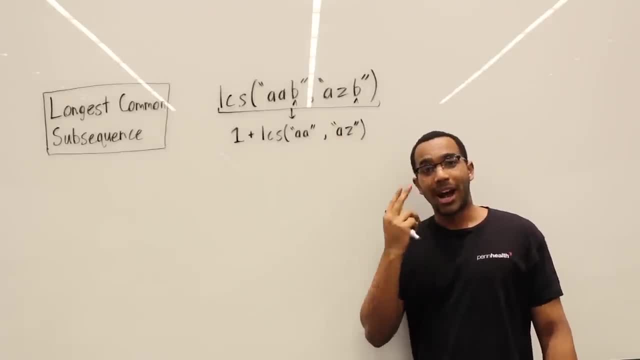 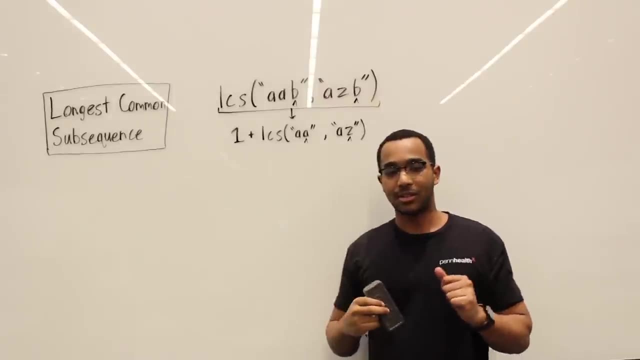 For these guys. And where do my eyes go? My eyes go to the last character. Are these characters the same? They are not the same. So my job now is is to see if I delete either of these characters. if I delete either of those characters, which which sub problem is going to yield me a better? 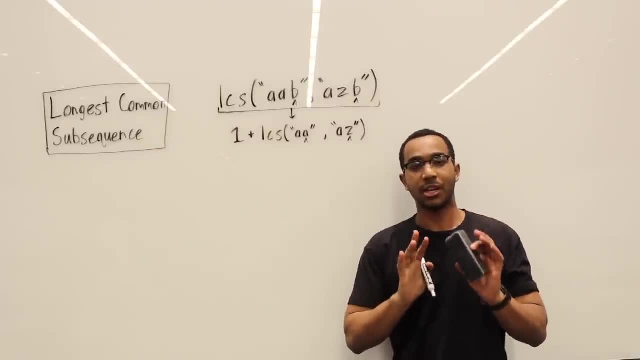 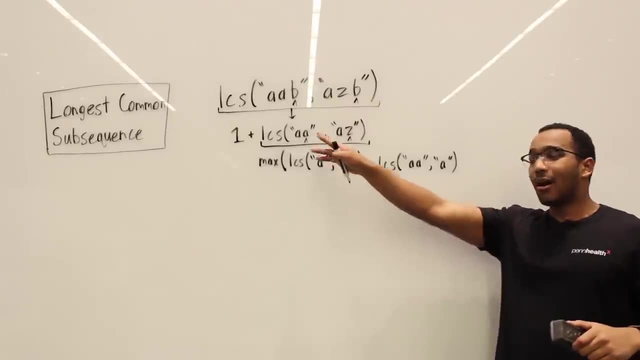 longest common subsequence. So stay with me, stay with me. It's confusing. Let me draw this out so that you can see. Okay, You see this now. So you can see how I broke this sub problem down into. if I remove this a and I 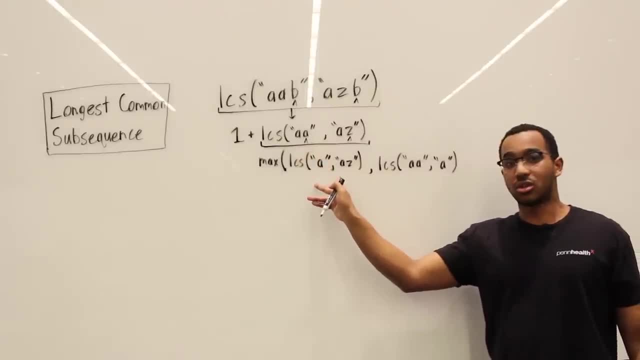 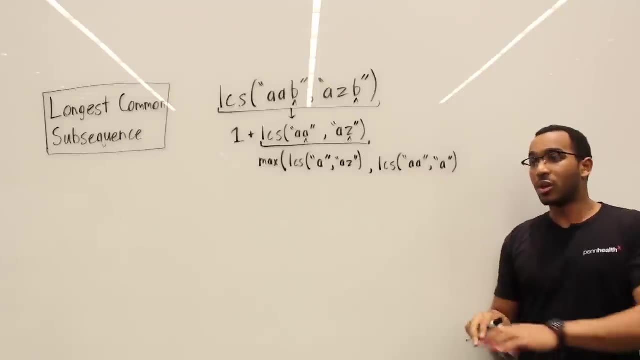 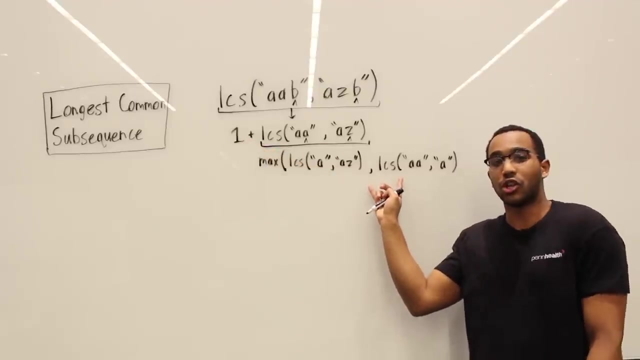 take the longest common subsequence between these two strings and then I remove the Z and then I take the longest common subsequence between these two strings. whichever of these yield a bigger longest common subsequence. whichever of these calls yield a larger answer, I'm going to take. 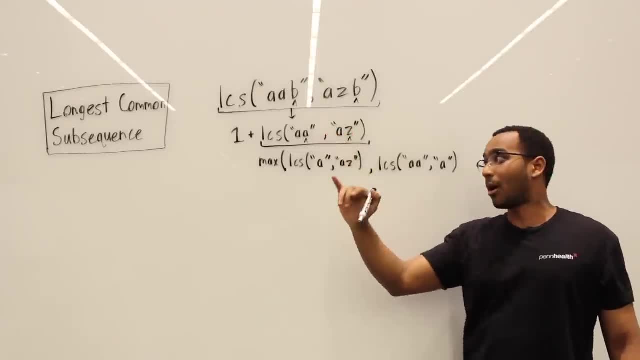 that as the longest common subsequence given this Sub problem, And then I'm going to add one to this in the stack frame. But the key here is: the best answer to this sub problem When we have mismatching characters is, I try, removing this character. I. 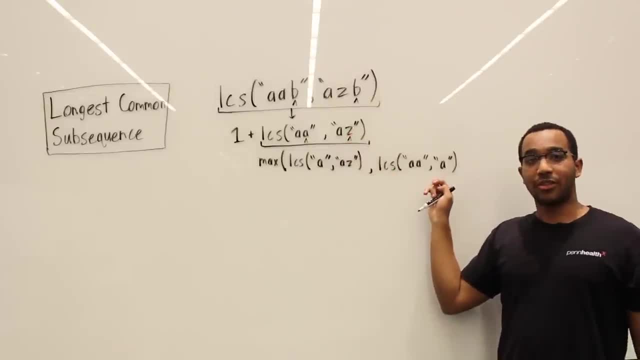 solve it. I try removing this character and I solve it. So this is confusing and we'll see it's less confusing when we get to the DP table. But what we're trying to do is we're trying to find the best sort of path to take in decomposing the string. 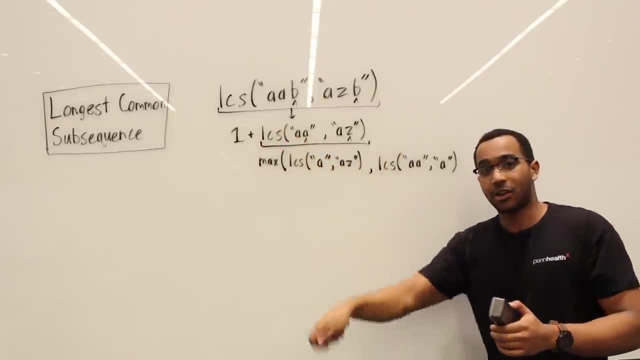 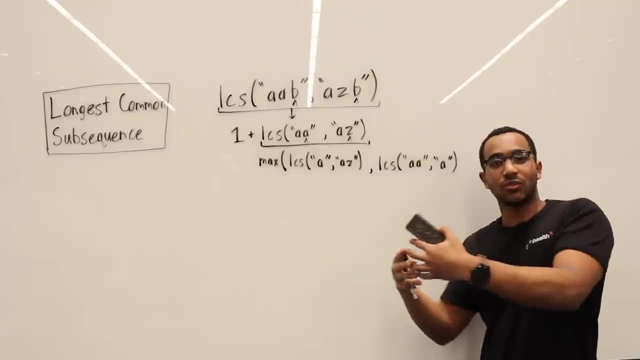 that's going to yield the longest common subsequence. And we're chopping off character by character, by character by character. We're cutting off characters and we want to see which combinations of chopping off characters is going to yield us the longest common subsequence. So how do these? 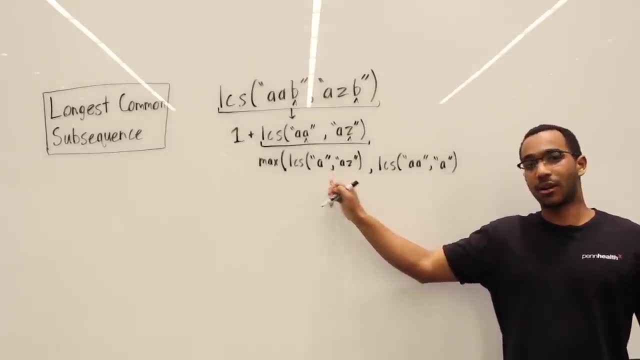 problems decompose. So this problem: we look at the last character, Are those a match? And we see that these guys are not a match. So this decomposes into the max of ripping this character off and ripping this character off, And then we're going to take the longest common subsequence and we're 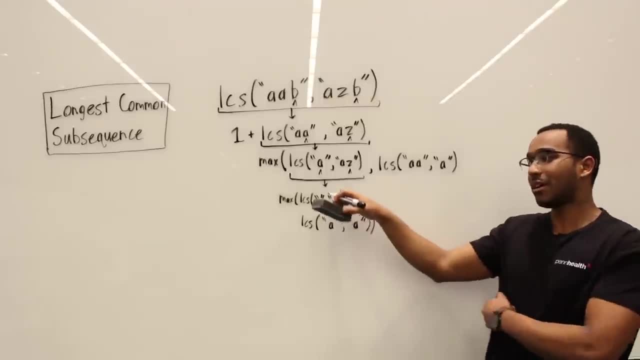 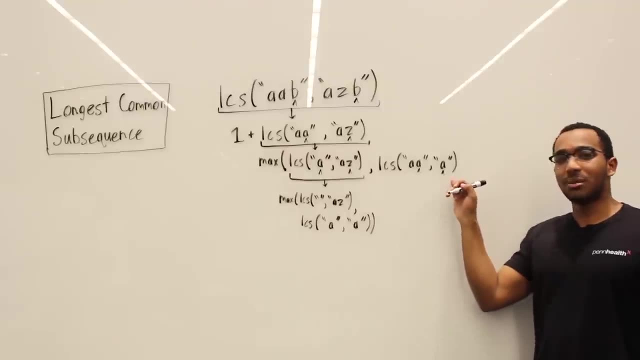 going to take this character off. So this is what it looks like. Okay, So that's how that decomposes, And then let's decompose him. Let's look at the last characters And then we see that they're a match. So what this means is, from this sub problem, this sub problem alone, this sub problem has no 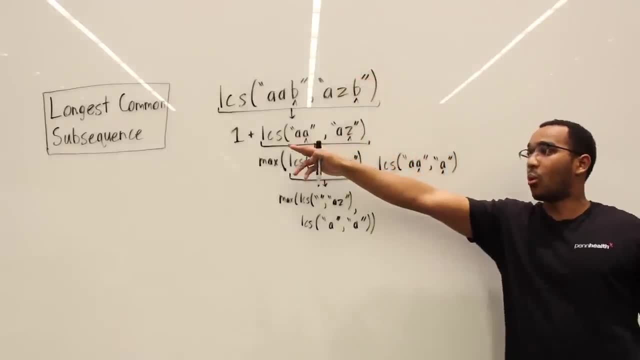 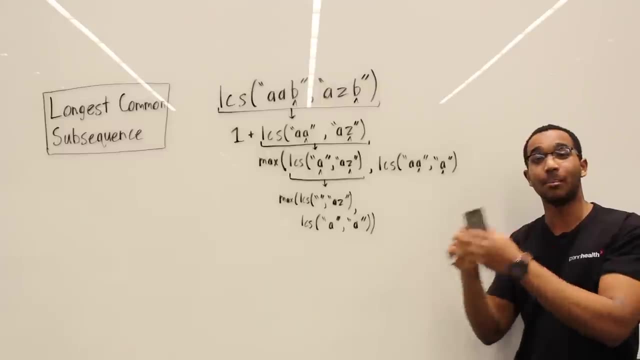 idea what's going on up here. What we can do is we can do the same thing, One plus removing this last character, because these guys were a match. There's no competition that needs to happen. We don't need to compete about whether we need to remove this guy or this guy. We can just. 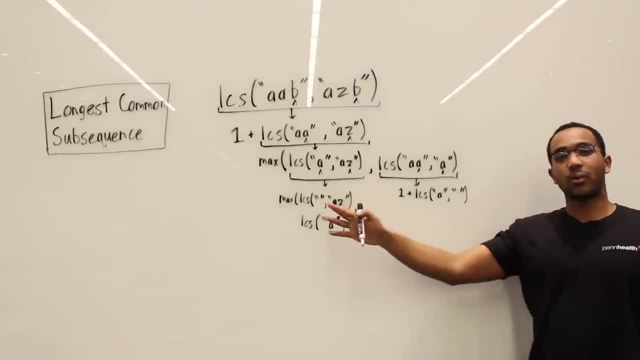 remove both because it's a match, Okay, So this is where our sub problems now stand, And you can see that this is kind of recursive in nature. So what we're going to do is what we're going to do is evaluate this guy. If I have the empty string and I have another string, if either of my strings 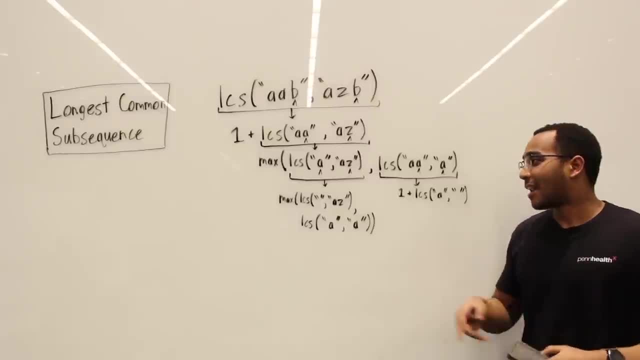 are empty. what does that mean? That means that there's not going to be a longest common subsequence. I can't have anything in common with an empty string. if that makes sense, I can't have anything in common between empty string and AZ. So the answer- the length of the longest common subsequence, is zero. 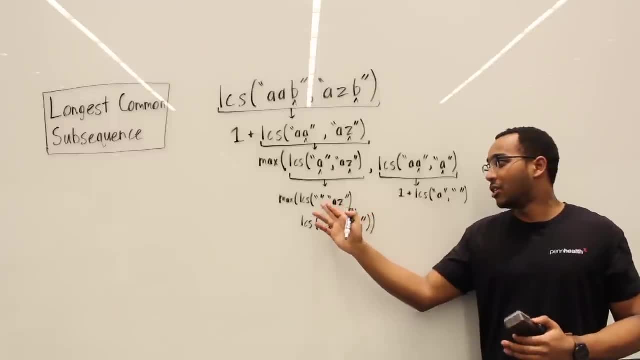 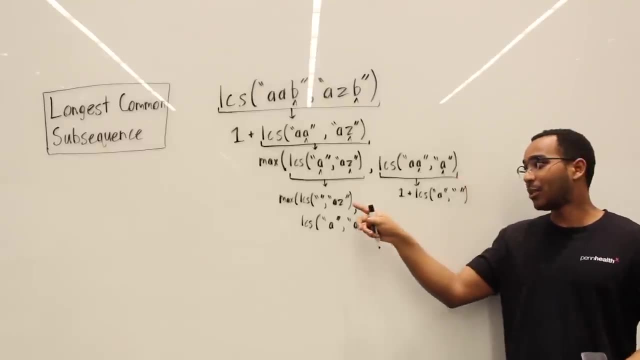 This is. there's no magic here. It just makes common sense that nothing versus something will have nothing in common. So we're going to put zero here. We've found a base case so we can evaluate this to zero. The longest common subsequence between these two guys is zero. Okay, And then 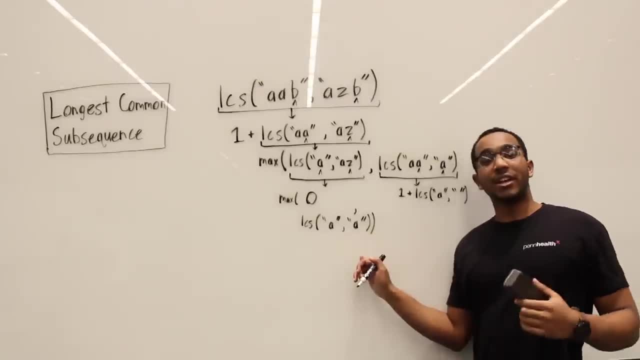 we can decompose this guy. And now what we can do is we can go downwards. And again, what do we do? We look at the last character and it's a match. And then we can decompose this guy. And now what? 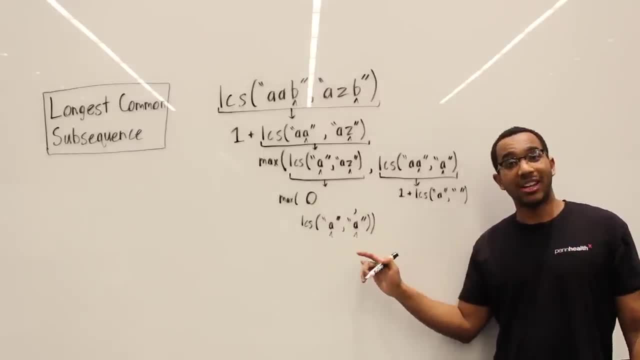 we can do is we can go downwards. And again, what do we do? We look at the last character and it's a match, So we do one plus removing both of these guys. Remember, no competition needs to happen. I don't need to do a max competition between removing him and him. I know that. I 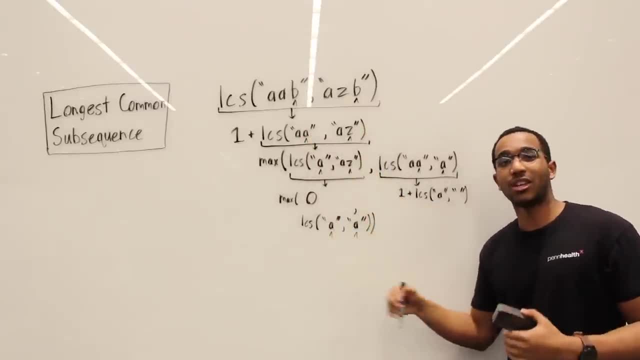 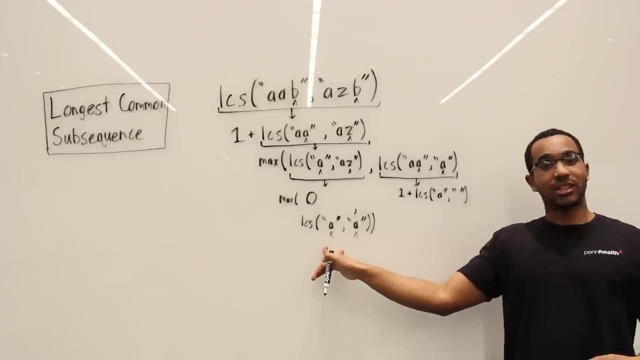 found a match, so these characters can both be removed, so I can do more work and I can evaluate against without these characters. So what happens is I turned this into this. Okay, So we found a match, we added one And now we're evaluating against without either character. We evaluate. 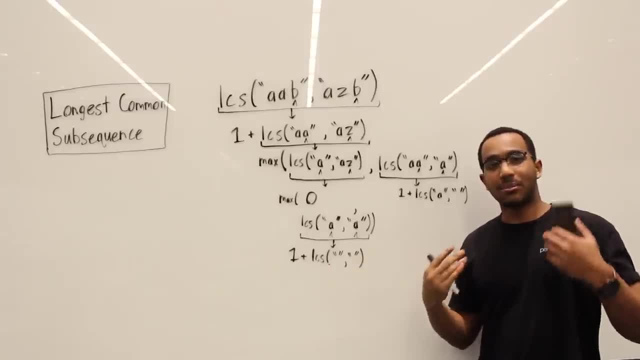 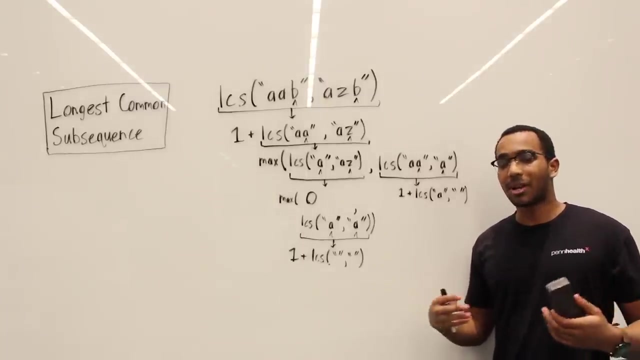 evaluate against empty string and empty string. Well, empty string and empty string will have a longest common subsequence of zero, because, empty string versus an empty string, there's nothing to have in common. If either of them are empty, we immediately have a longest common subsequence of zero. 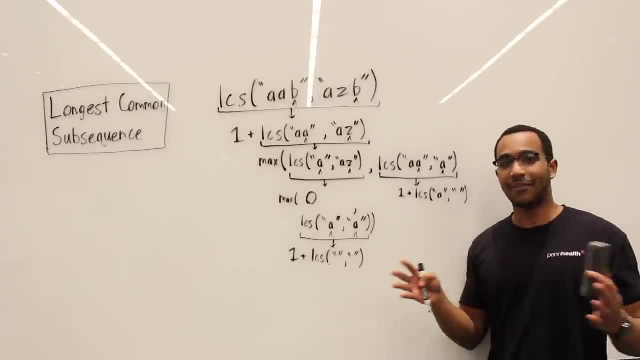 because an empty string cannot relate to anything, It cannot have a shared subsequence, It has nothing. So what we do is that becomes zero. So again, we're not tracing the recursion exactly, because this can be modeled recursively, but we have one plus zero and we can evaluate this guy. 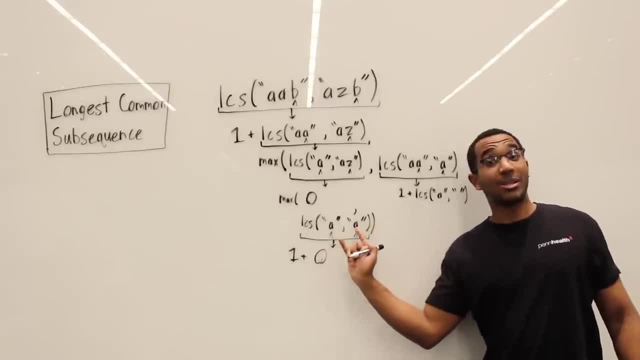 This guy becomes one And notice the longest common subsequence between A and A is one, The length is one, And notice that's true, A and A are a shared common subsequence, It's one, so that makes sense. So what is the max of zero and one? 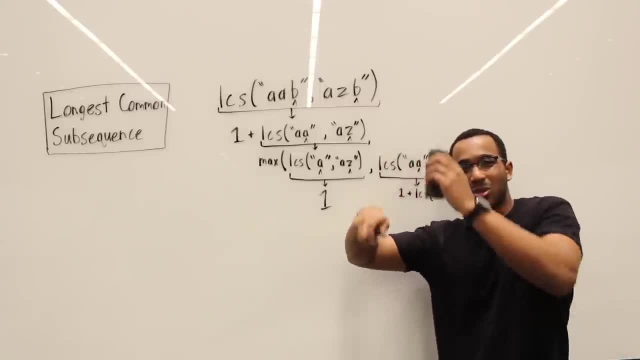 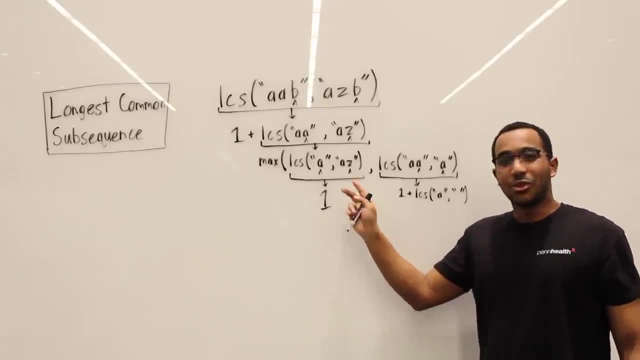 It's one. So do you see here, do you see how we're drilling down, sub-probleming down until we get to solid answers? So our solid answer here is one. So do you see this sub-problem A versus AZ. 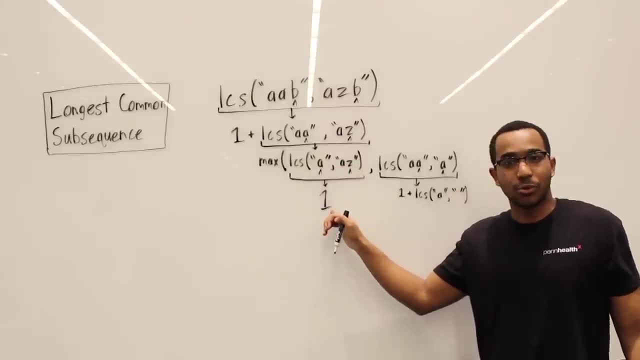 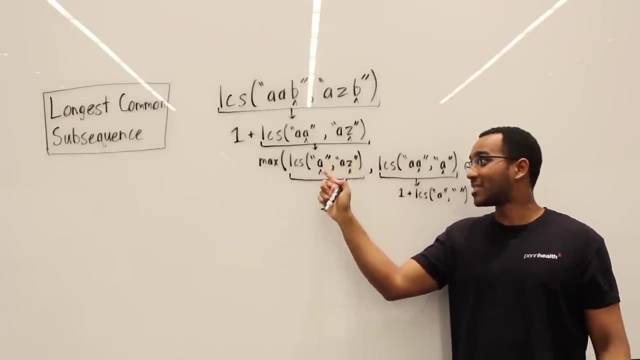 The answer to the sub-problem is one. Is that true? And it is true. A and A are matching, They match, and that is the longest common subsequence: A and A. The answer to the sub-problem is one, So let's materialize that. 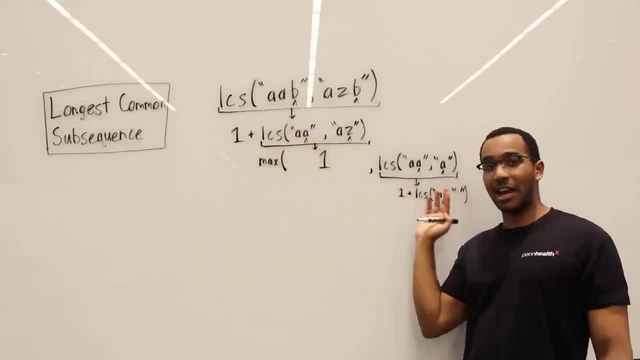 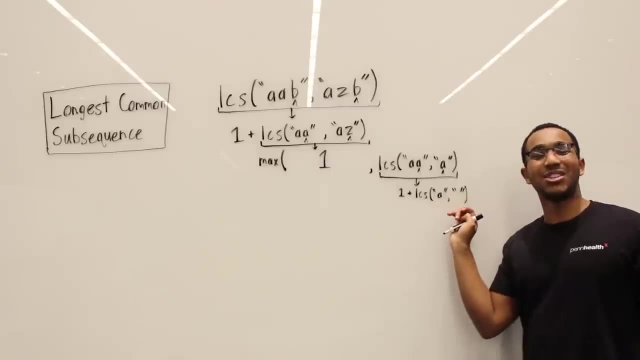 So what's happening is, this sub-problem is still being worked on down here. We've materialized this guy, So let's work over here. So what is the longest common subsequence between an empty string and a character? Remember, if I have an empty string. 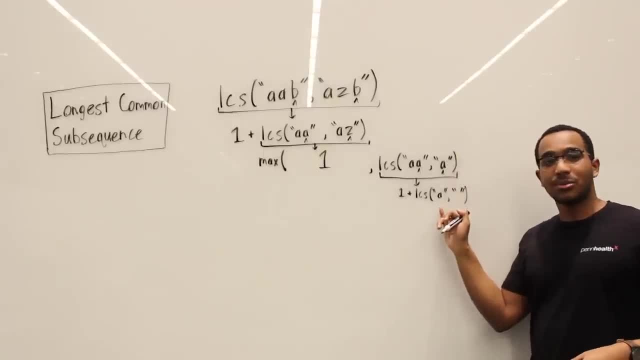 I can't relate to anything. So what happens is this becomes zero. One plus zero is one. And is this true? The longest common subsequence between A, A and A is it one? And yes, it is one. Do you see? 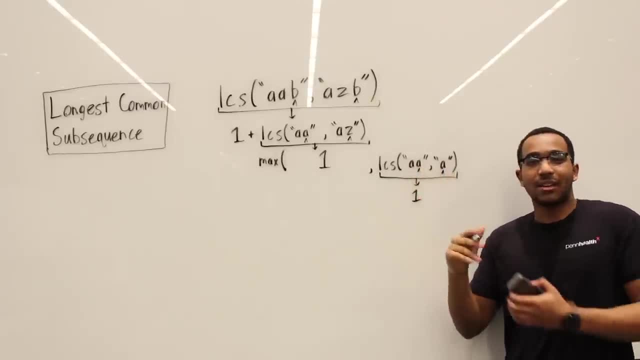 We either can match those As, or we can either match A to A. We're limited by one A, so it can only be one. So what we see here is what we do, is we evaluate that to one. That is the answer to the sub-problem, right here. 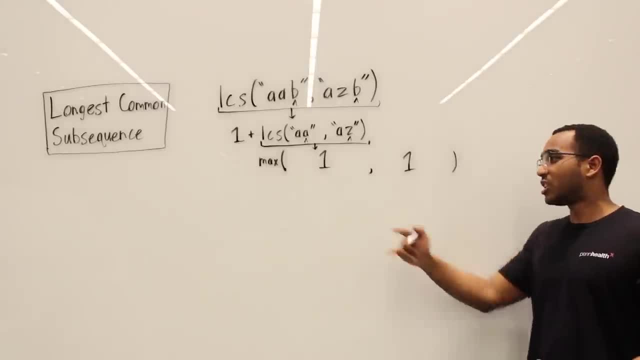 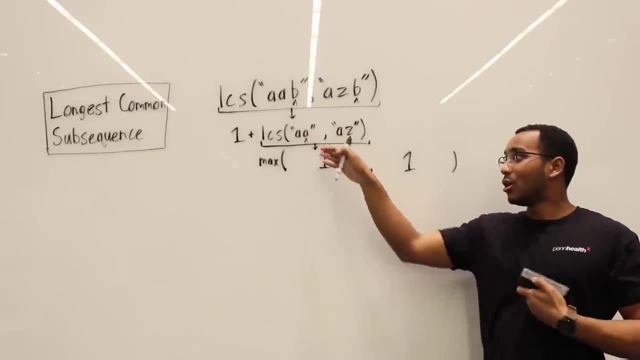 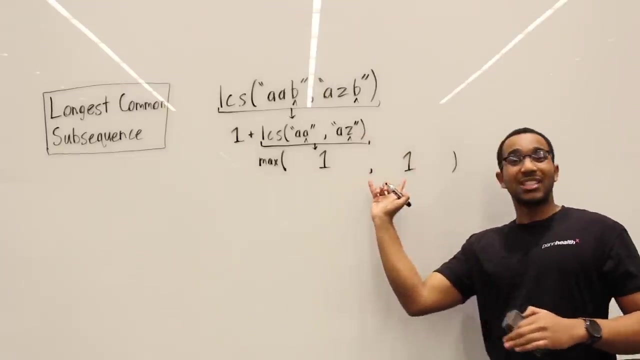 So we have our competition. Our competition is finished. We tried removing him. We tried removing him. The yielded answer from removing him was one. The answer yielded from removing him was one, or I may have swapped that, But do you see? 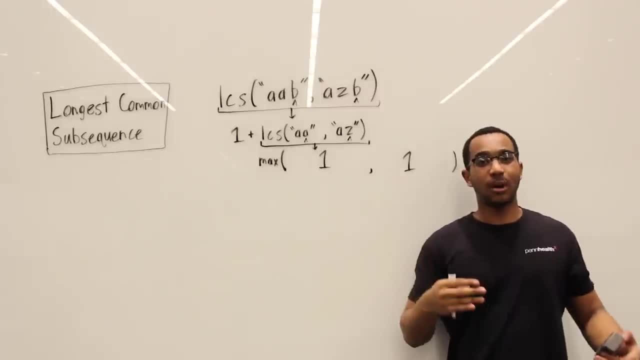 We're competing and the competition is one by whichever sub-problem is going to yield a longer common subsequence based on who we chopped off because these guys didn't match. If they did match, we would chop both of them off, But because they did not match. 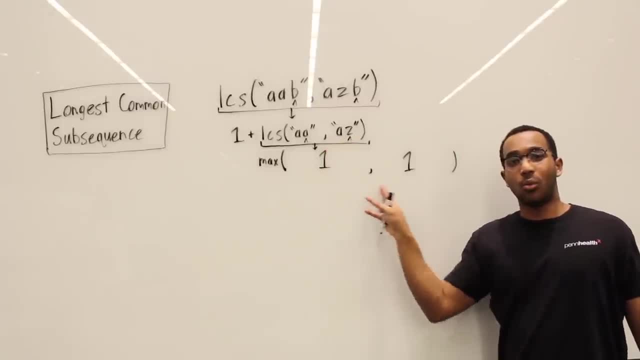 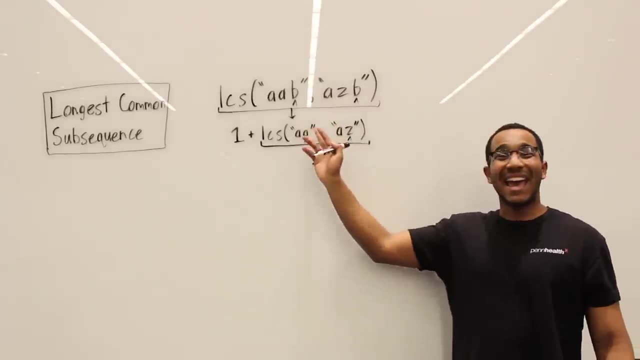 we had to do a competition. So what we see here is one and one. What's the max of one and one? It's just going to be one. So what is the length of the longest common subsequence between A, A and A Z? 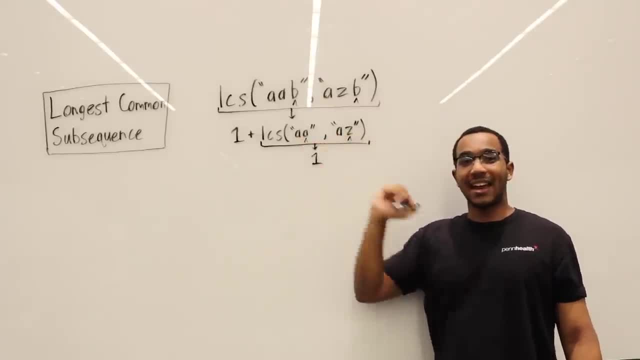 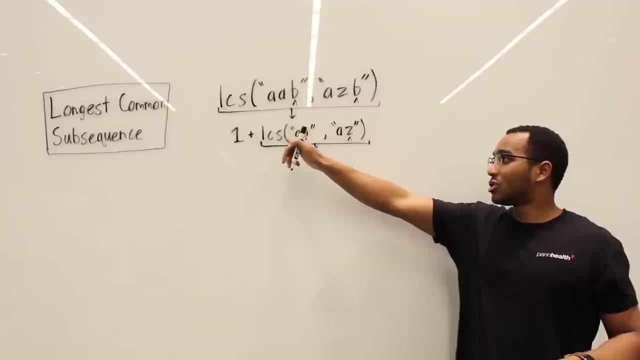 Do you see how it's one? Do you see how we can match this A to that A? Or we can match the final A in the first string to this A. All we have is this A to play with over here. So the answer to this sub-problem is one. 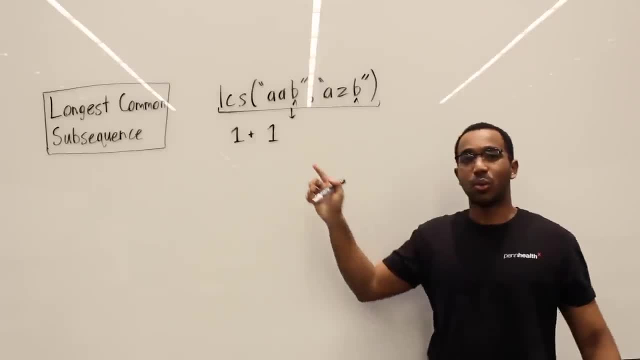 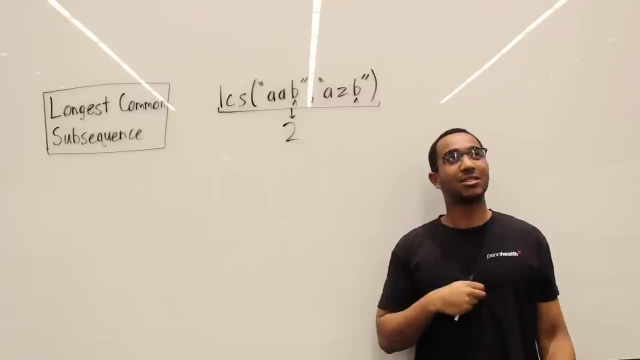 The sub-problem's answer is one. And what is one plus one, Two? And this is the magical thing about this- Our answer is two. Is that true, Am I right? So look at these strings: A, A, B and A, Z B. 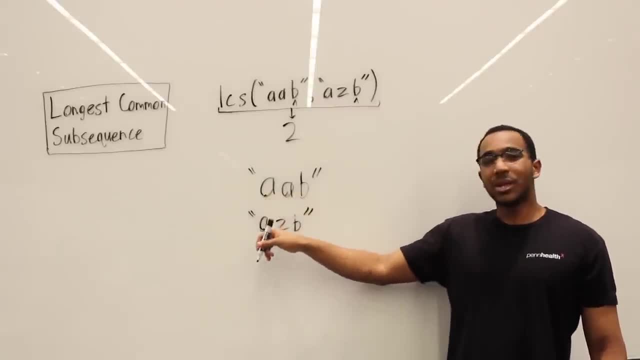 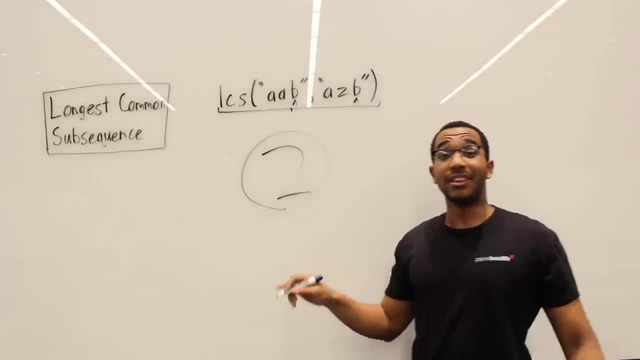 So what we see here is A, A, B, So we can see, we can match the As, and then we see the Bs match. And what is our output? Our output is right there. The answer to this overarching sub-problem is two. 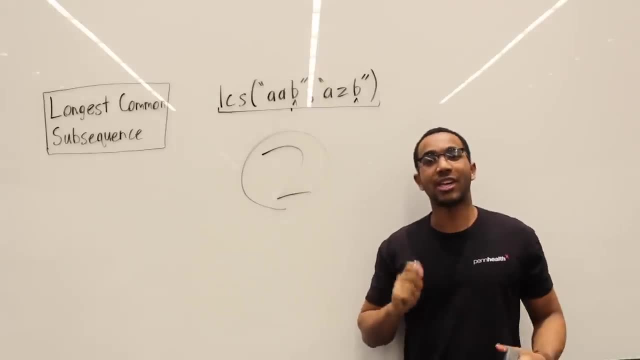 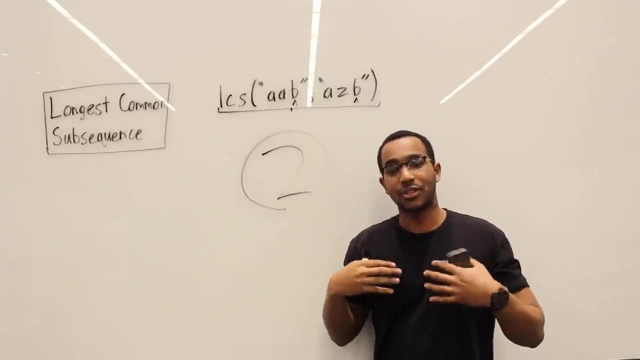 And I want you to know that when I did this walkthrough, I did not look at any code, I did not premeditate this. I literally just wrote this on the board And, from my understanding of how this problem fundamentally decomposes, I just wrote the recursion. 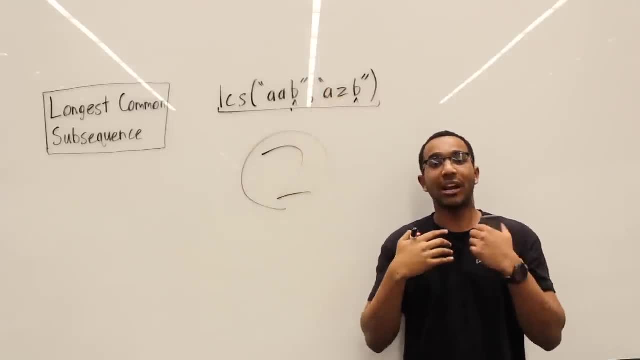 how the recursion would pan out and we got our answer. So this is what I want to communicate to you. Yes, we can memorize problems, We can memorize how to do certain things, But if you have a real deep understanding of how these sub-problems caught up into each other, 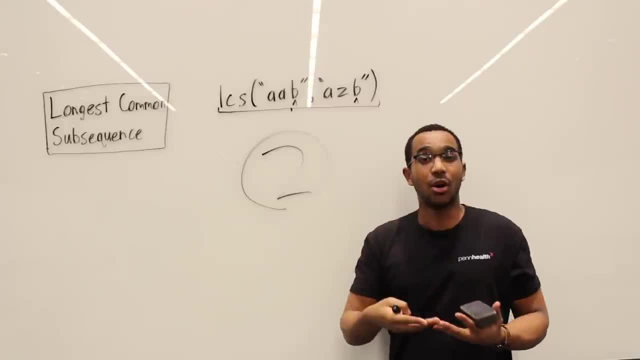 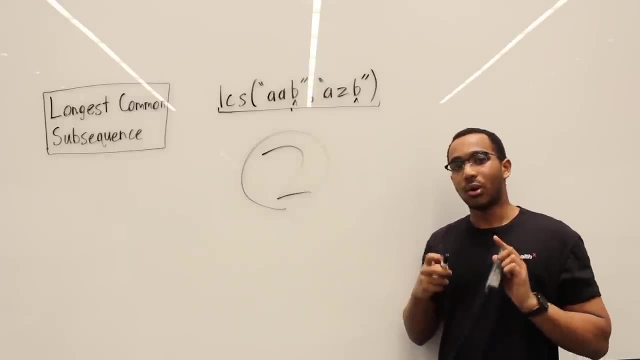 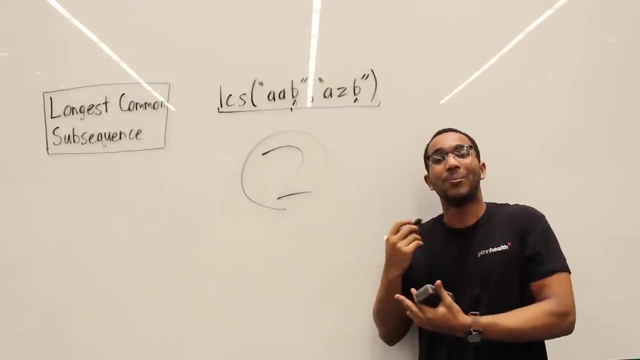 then you can do this problem without needing to see the code And then it becomes easier to go into implementation with understanding. So what we're going to do now is we're going to look at the dynamic programming table to really reinforce what this idea of sub-problem. 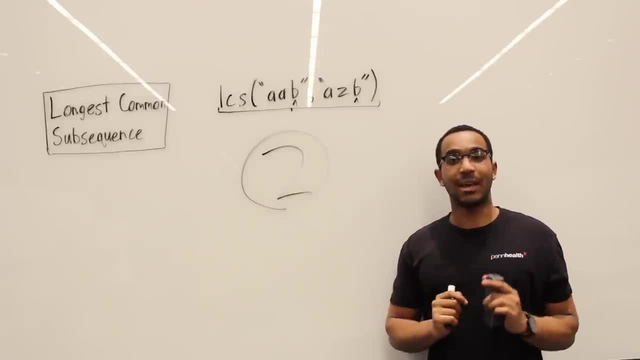 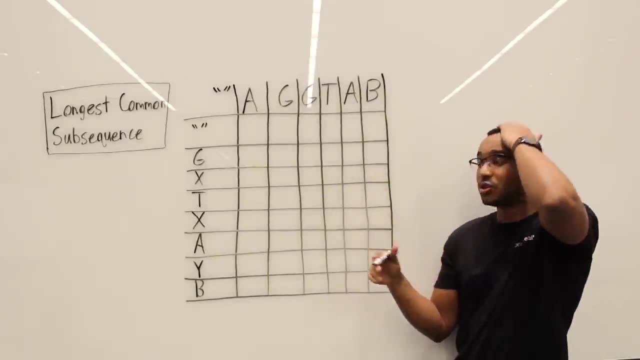 decomposition is all about. So let's look at that table right now. OK, So what I'm going to do here is we're going to walk through the dynamic programming table and how we would do this to cache sub-problems. So this problem is very similar to the Levenstein distance. 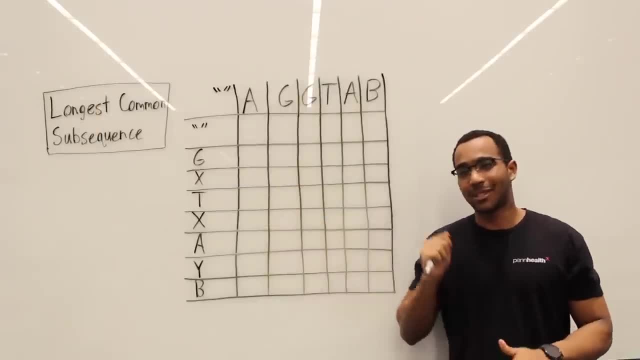 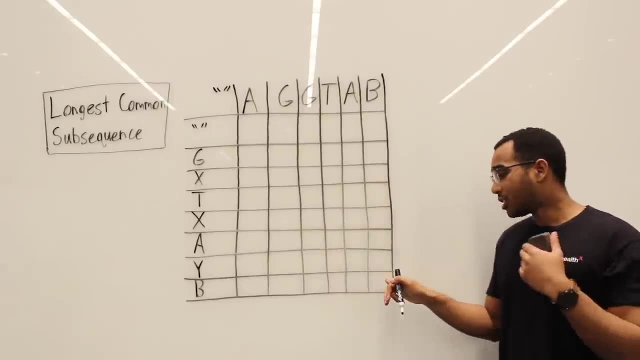 I have a video on that And I really feel bad because I was not completely clear about what each of these cells meant. It is very, very simple. What does this cell mean? That cell right there means this. So do you see that right there? 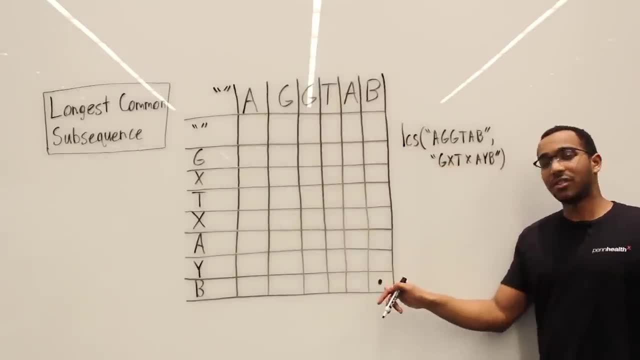 Do you see how it is a function call. All each of these cells means is a different substring chopping that we call this function on. They're sub-problems. What I'm doing here is not different at all from what I just did in the walkthrough that I showed you. 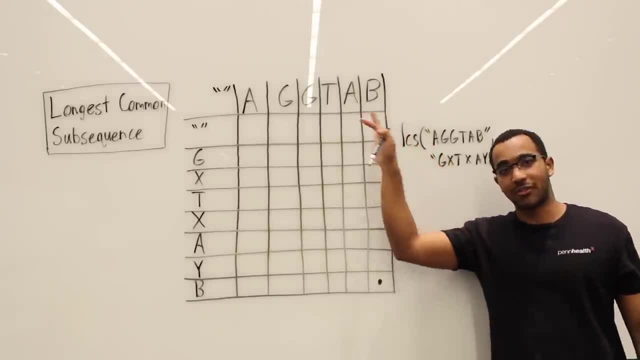 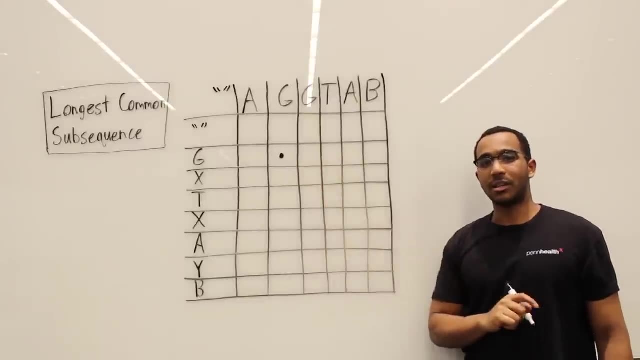 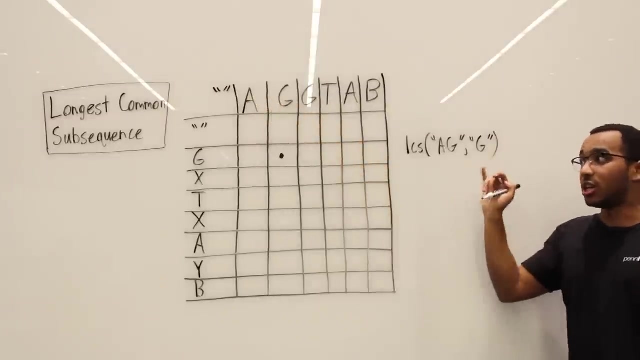 It's just we're formalizing this because our code will have to iterate and store stuff in a table. So this is what that cell right there means. What does this cell mean? What does that cell right there mean? It means this: It means the sub-problem: AG, AG and just the G, just the G. 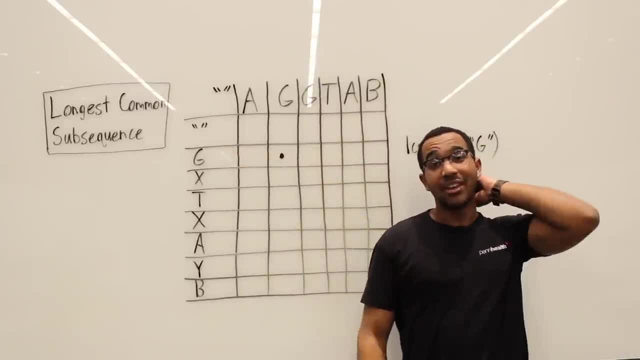 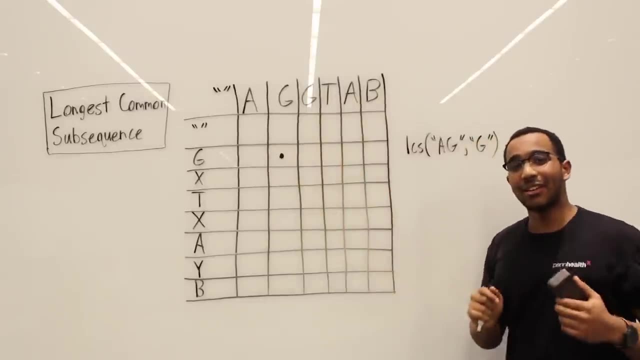 So that is what it means When I'm breaking these into sub-problems. they're separate function calls. They're separate function calls we're breaking things down into. So the key here is to understand our sub-problems. So let's define our base cases here. 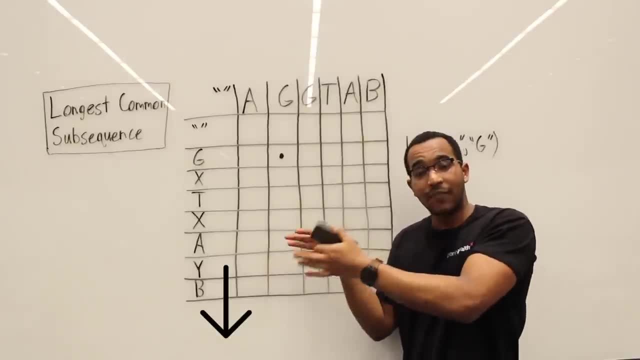 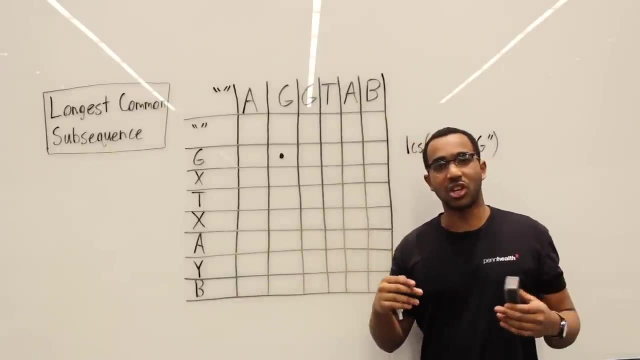 This is not how the code would do it, but code is in the description. If you want to see the concrete implementations, I have put it there. The code is in the description, But I'm going to walk you through this, just as you know. 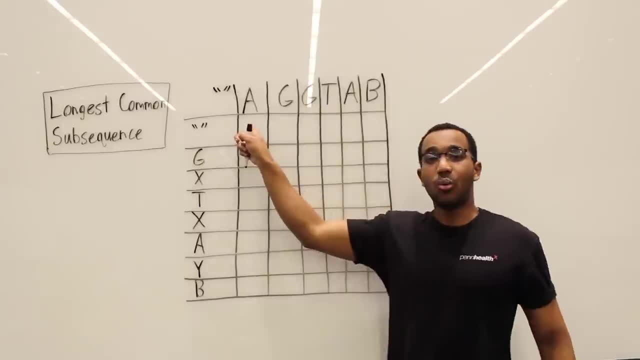 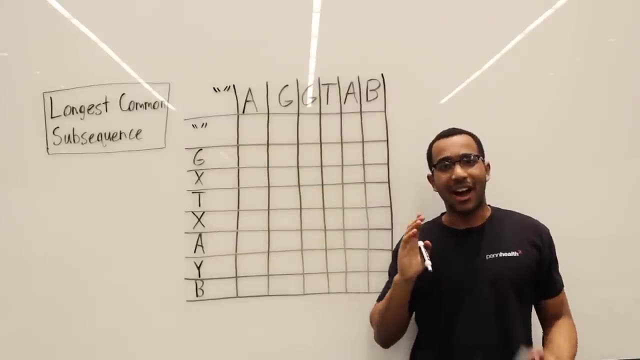 you would normally think about it. So let's see how that goes. So we have A versus an empty string. What is the longest common sub-sequence? Remember what I said: If either is an empty string, they cannot have anything in common. 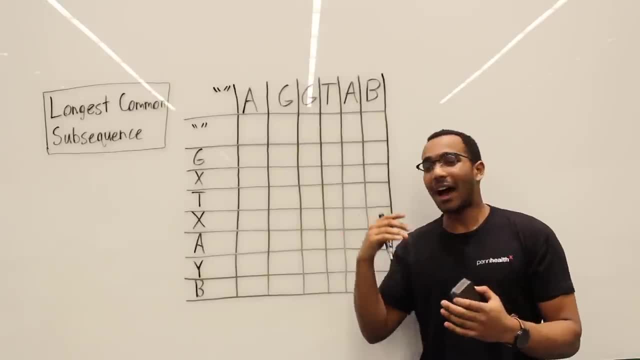 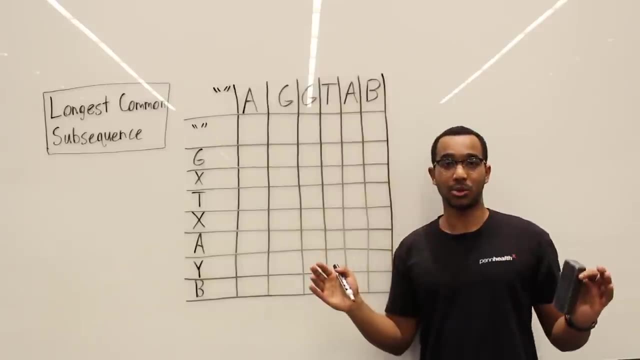 An empty string cannot share anything. It does not matter what string you give me. If I have an empty string, I cannot find it. I cannot find any common sub-sequence between them, because it's an empty string. So this is going to be zero. 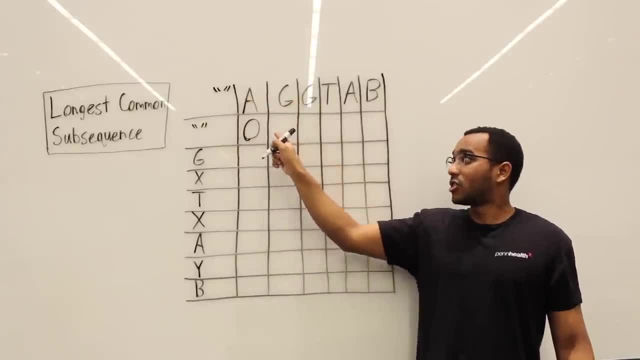 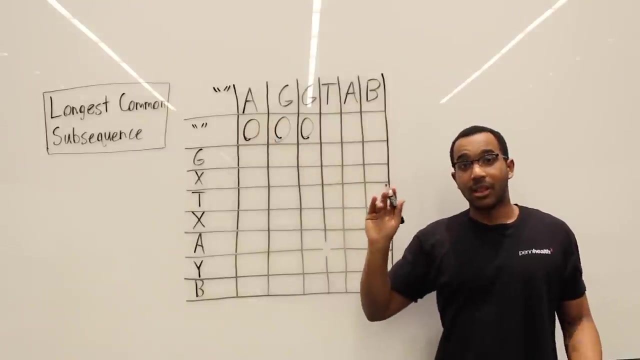 And then A G A G versus an empty string- Again zero. And then A G G versus an empty string- zero. And then A G G T versus an empty string- That's going to be zero. And then again we're going to compare. 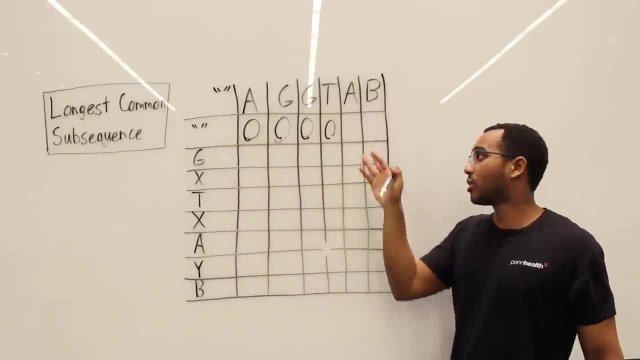 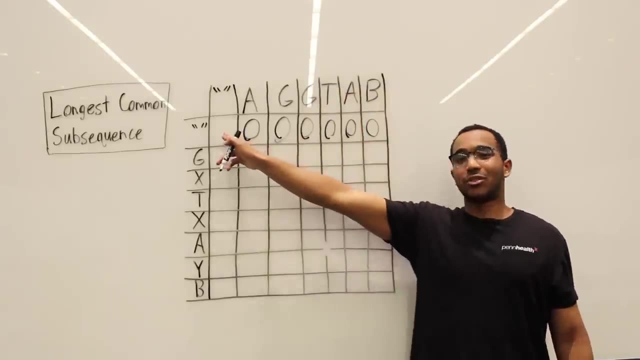 against an empty string. We're going to call that LCS function on an empty string: Zero and zero. Okay, I just realized I forgot a column right there, My bad. So yeah, empty string versus an empty string, that's going to be zero. 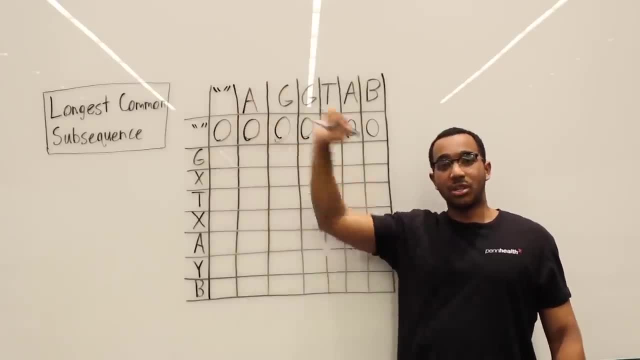 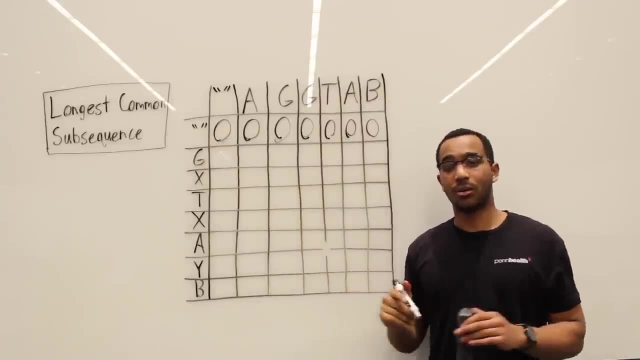 Okay, so now we're back to normal. So G versus an empty string- Anytime I'm comparing against an empty string, what is the answer to the longest common sub-sequence problem? Zero, G, X versus the empty string, Zero. 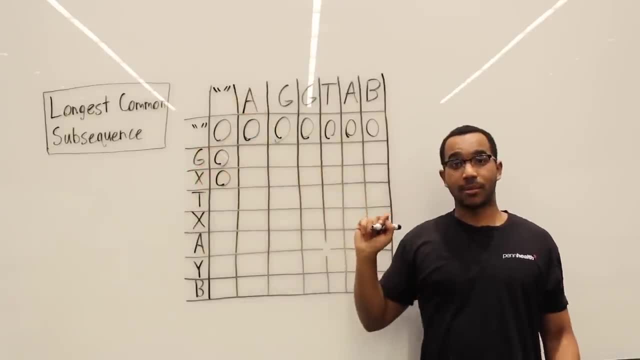 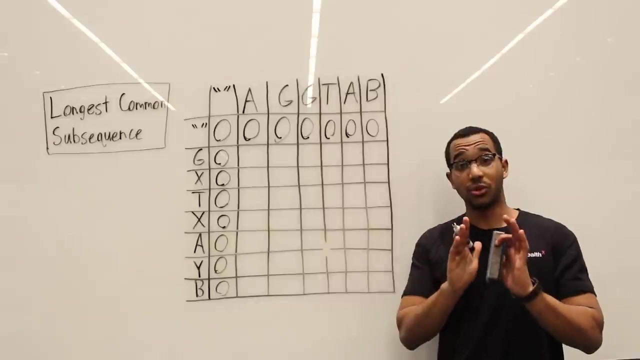 G X, T versus the empty string: Zero. G X, T, X versus the empty string: Nothing in common. So the rest of these guys, compared against an empty string, are zero. Okay, so now the work begins. So what we're going to do is: 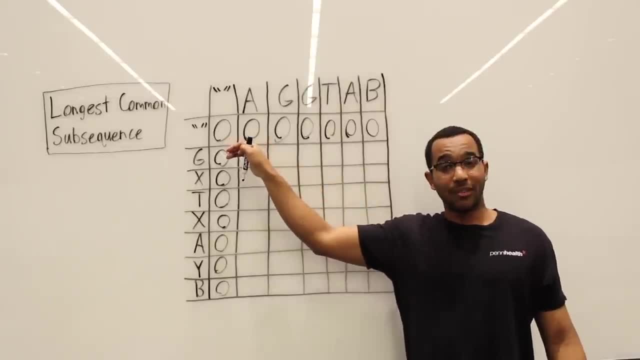 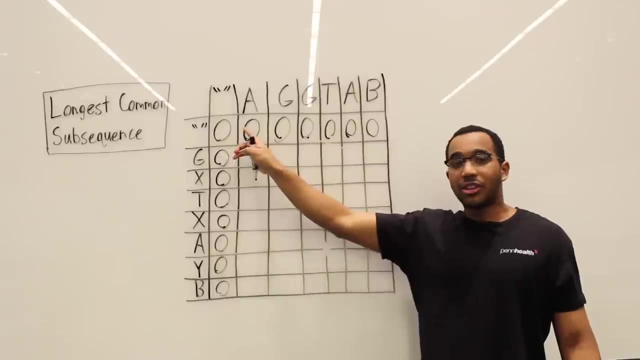 what I'm going to do is I'm going to see: are these characters equivalent? I'm going to do a normal iteration, row by row, column by column, like that, And what I'm going to see is at this cell: are these characters the same? 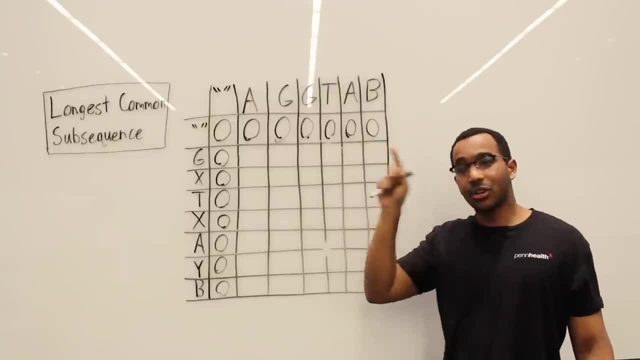 A and G. Remember how we cared about the last cell, The last character. We're caring about the last character here. These characters are not the same. So what I do is I compete, I remove the A If I cut the A off. I'm going this way. 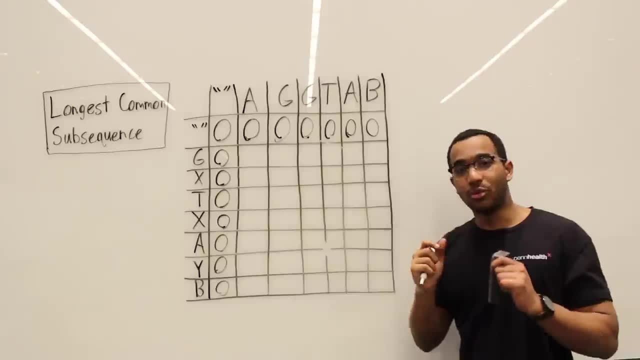 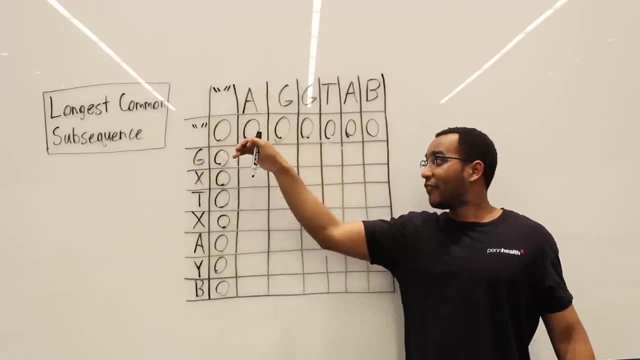 If I cut the G off, I'm going upwards, if that makes sense. If you really understand what's happening in terms of our substring matching here, we see that we're comparing A to G. If I want to remove G, I just go up and cut it out. 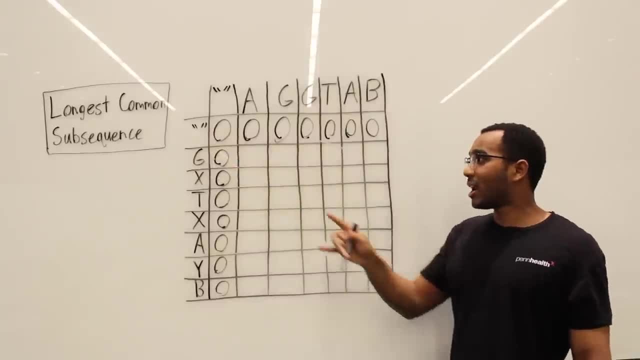 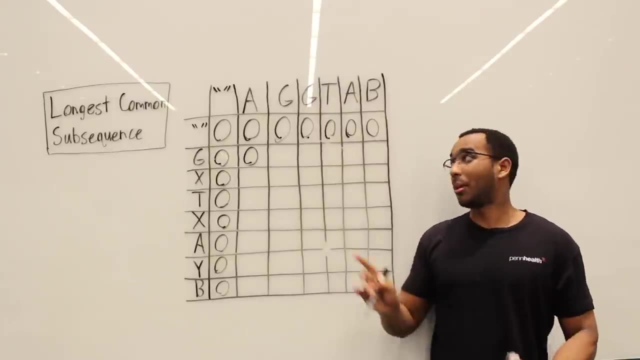 If I want to remove A, I just go this way and cut it out. So what I do is: what is the max of zero and zero. So the answer is zero. So the answer to the subproblem of A compared to G is zero. 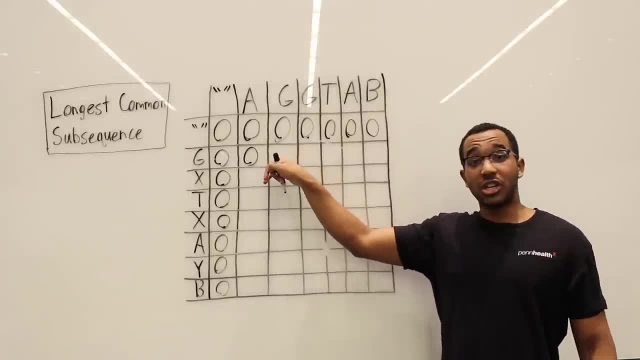 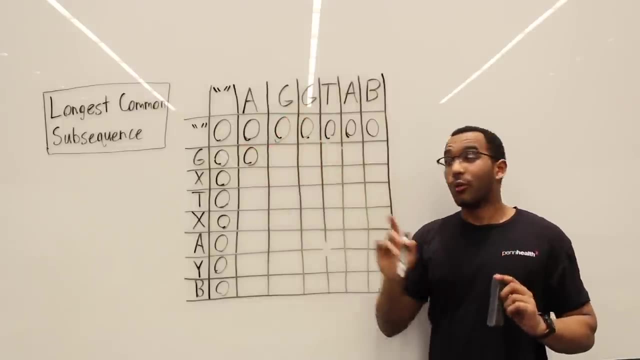 So what we do is we continue our iteration G versus G. We have a winner, So G is the same thing as G, So we do one plus removing both of these characters. How do I remove this G Go up. How do I remove that G? 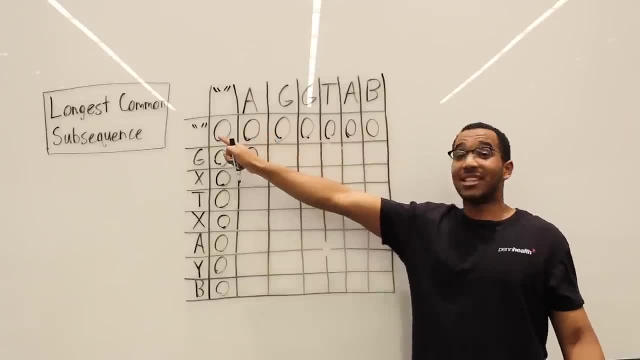 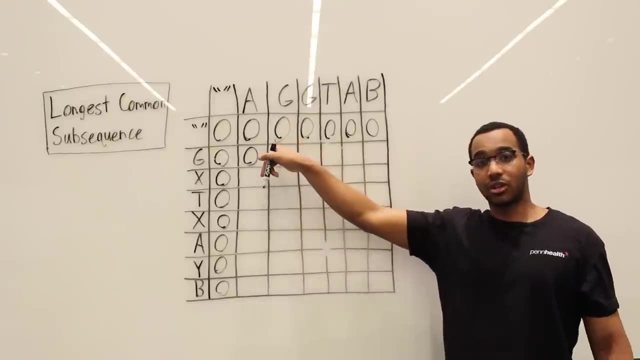 Go to the left And now our subproblem is the empty string and A, So we do one plus the answer to this subproblem, And that is the answer to this subproblem. Remember, what we're doing right now is not different at all. 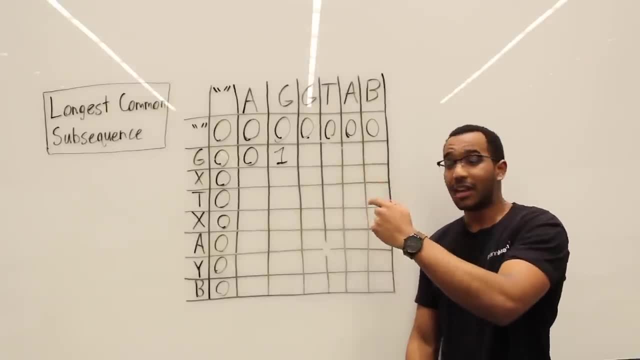 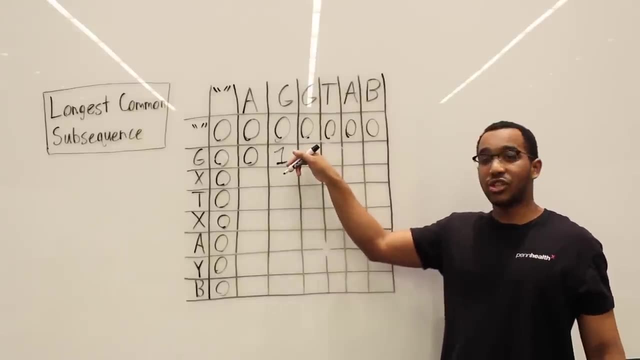 from what we did in the beginning. The beginning was the understanding. Now this is just how we would implement it and do comparisons in a bottom-up manner. So what we do is we compare G and G. It's a match. We go here. 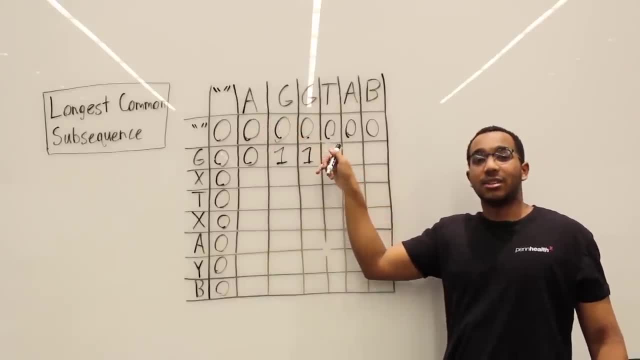 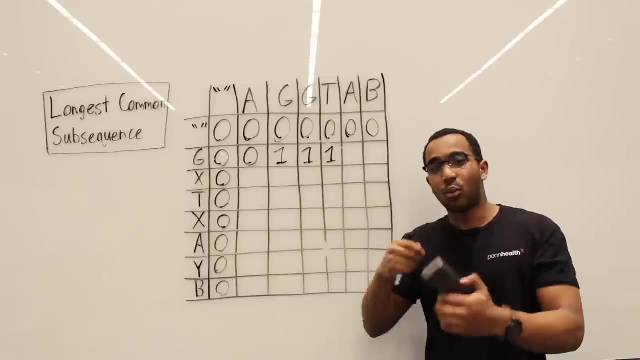 One plus zero is one G and T. That's a mismatch. What is the maximum? item One: And the reason I'm speeding up here is because the understandings were nailed down in that initial portion where we talked about the recursion and I talked about the subprobleming. 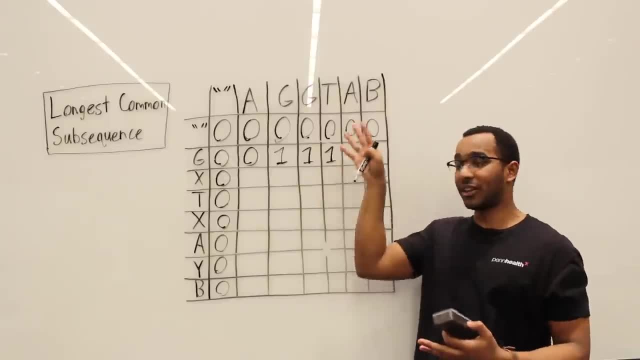 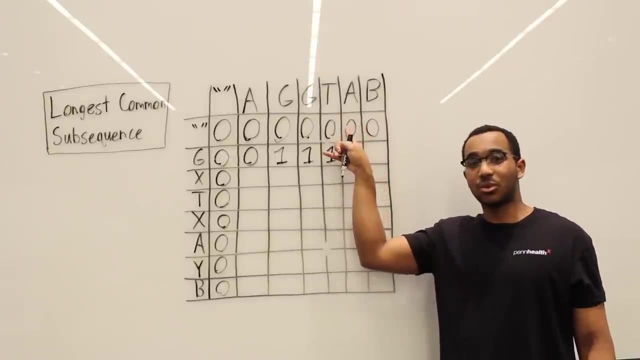 Now we're just worried about implementing this and getting things going in terms of filling this table out. So now A versus G mismatch. I want to compete subproblems. What's the max of these two guys? One, Okay, so now I have B and G. 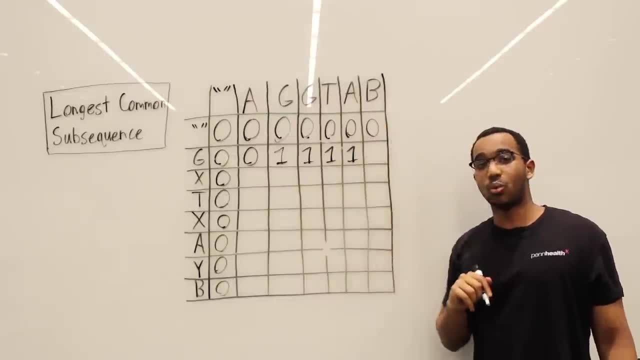 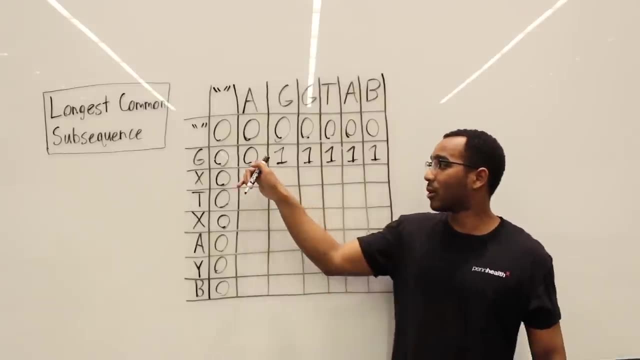 They're not the same thing. We compete subproblems. The max is one. Okay, so we're just gonna continue like this and our answer to the grand subproblem will be down there. So it's very straightforward: X and A mismatch. 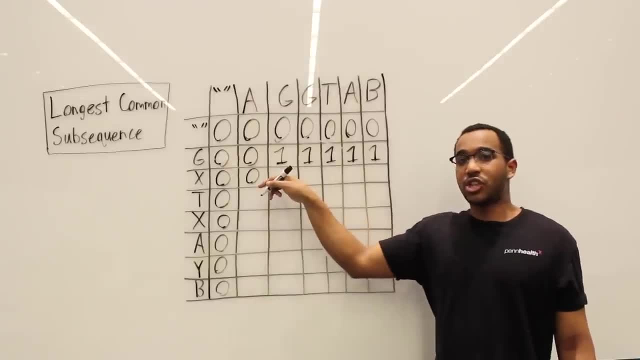 We put zero here. The max of these two guys is zero. X and G- These are mismatches. The max of these two guys is one. G and X mismatch, The max is one. T and X mismatch, The max is one. 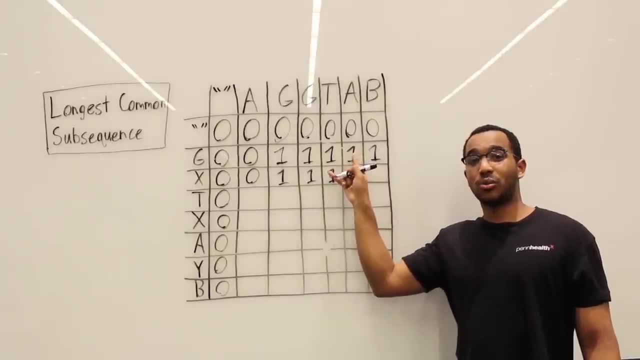 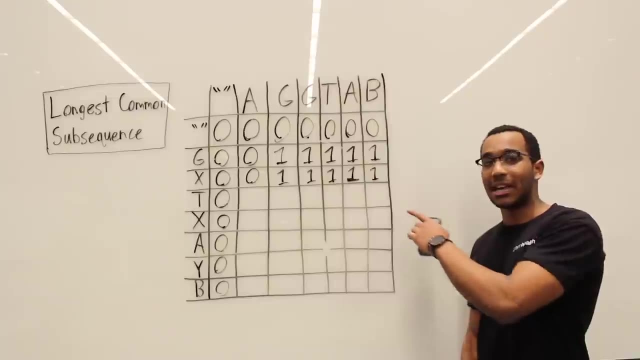 A and X mismatch. The max is one between these two sets, The max between these two cells. And then B and X. The max between these two cells is one. And again we did that because that was a mismatch. So onto the next row. 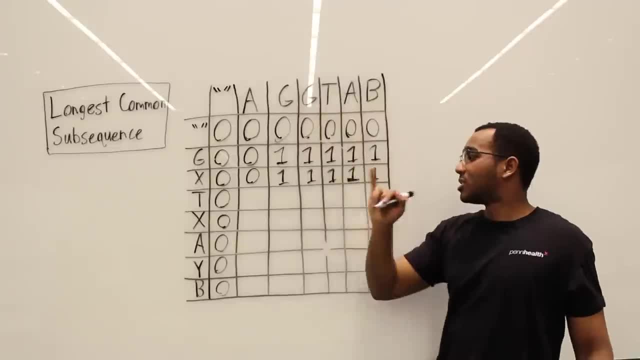 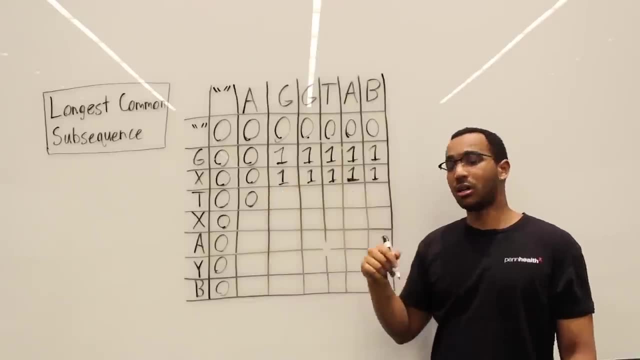 We see that mismatches happen all the way up to the T, So we're gonna take a max here. The max between zero and zero is zero. The max between one and zero is one. Again, G is a mismatch against T, One and one. the maximum is one. 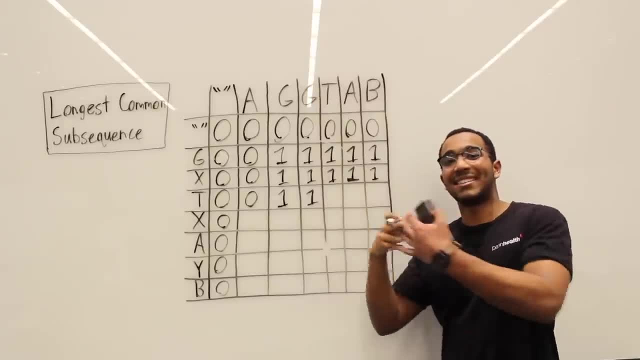 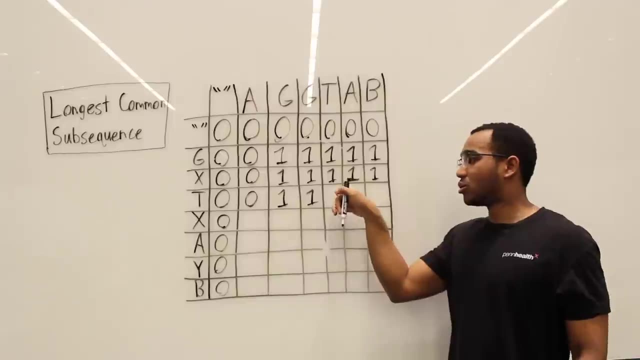 And then T and T. We have a match We can extend And the longest common subsequence between the T's removed if we remove the T's. So to remove this T, I go up. To remove that T, I go to the left. 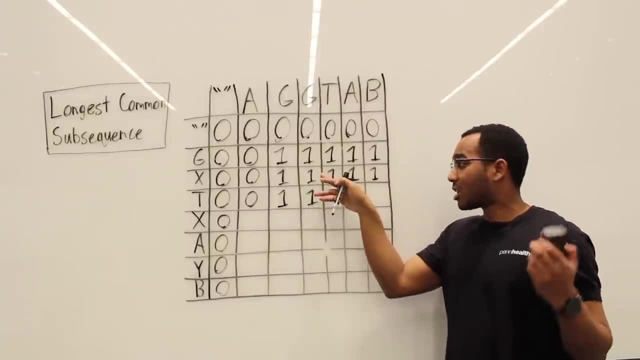 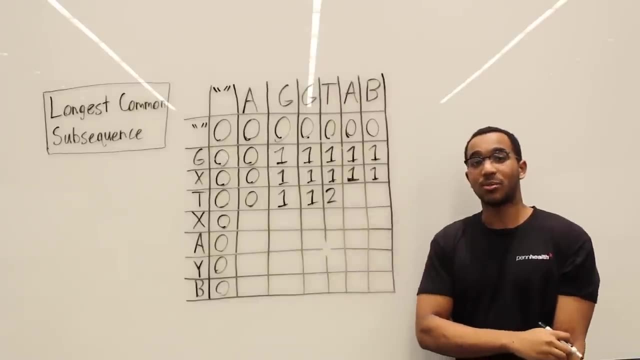 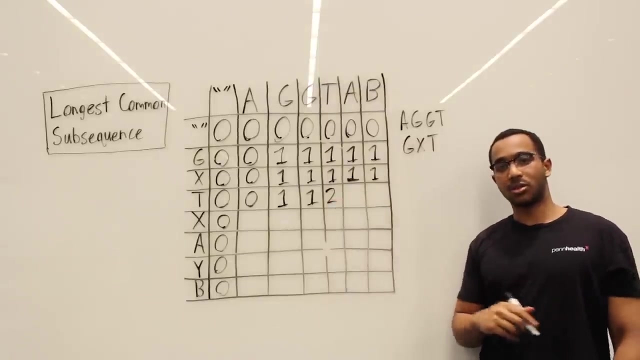 And I have a subproblem answer of one, One plus the subproblem answer here, with the T's removed, is one plus one, which is two. So the longest common subsequence between AGGT and GXT. what is the length of the longest common subsequence? 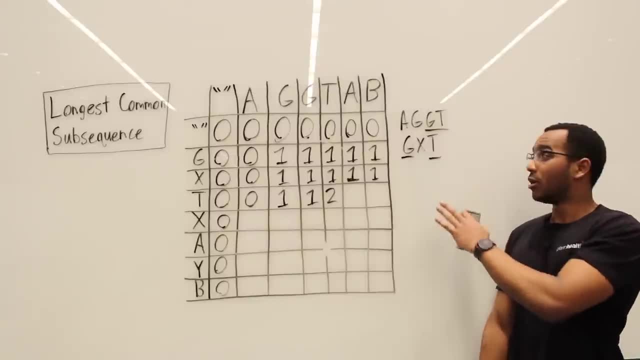 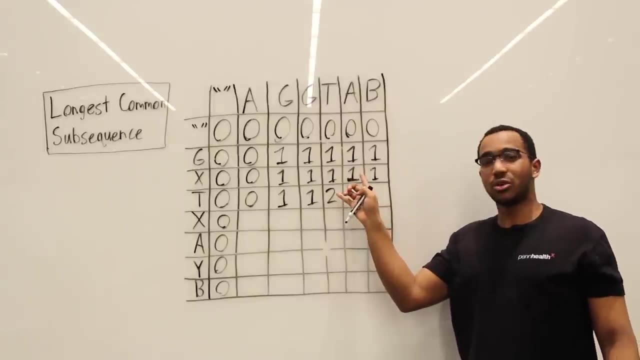 It's two And as you can see for a fact, it is two. Right there, you see, there's the longest common subsequences that match up there. So the T and A it's a mismatch. We need to do a competition. 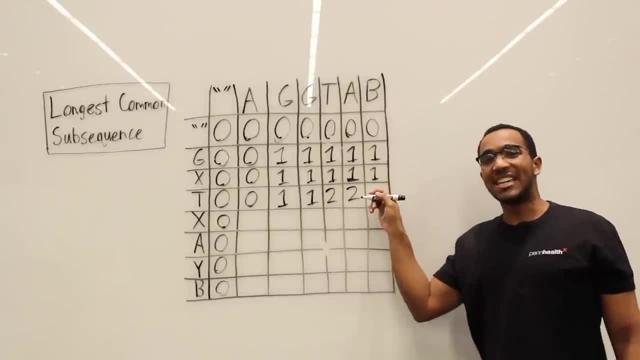 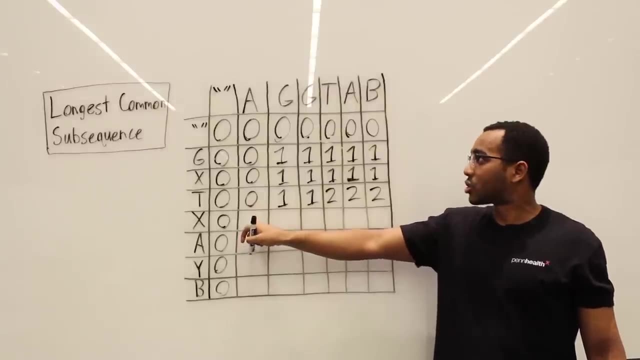 Who's the winner? The max of two and one is two. So T and B is a mismatch. The max of two and one is two. Onto the next row: A and X mismatch. So what we need to do is max of zero and zero is zero. 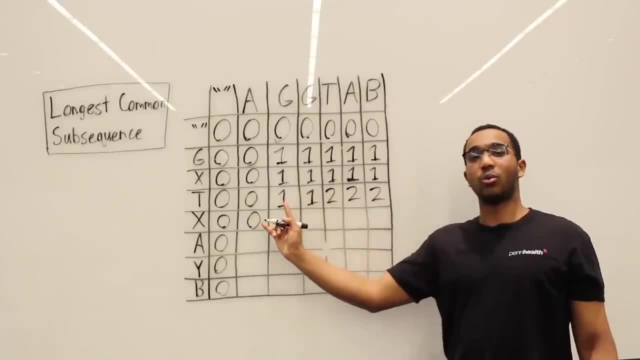 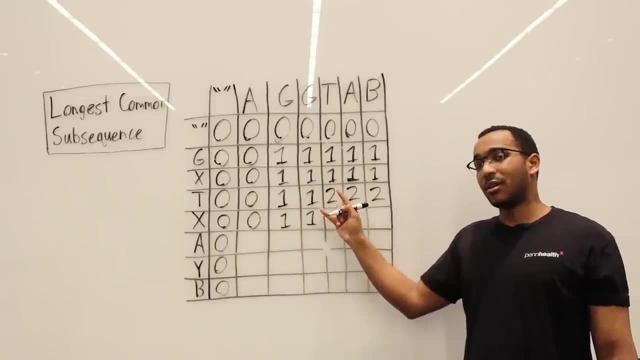 G and X mismatch, The max of zero and one is one. G and X again mismatch One and one. the maximum is one: T and X. it's a mismatch. The max is two between two and one. 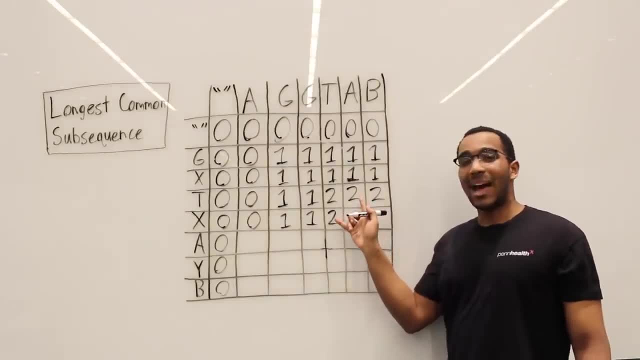 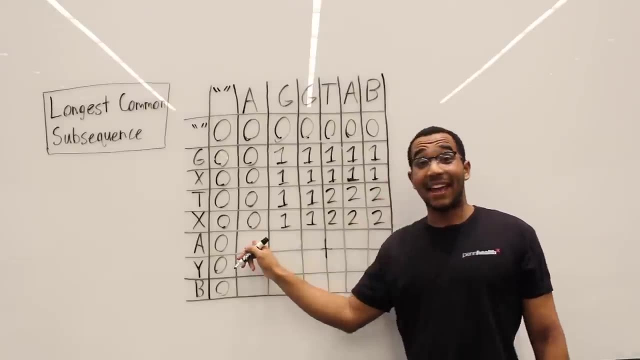 The max is two: A and X: a mismatch. The max between two and two is two, So B and X. it's a mismatch. So two and two. the max is two: A and A. we have a match. What we do is remove the A, remove the A. 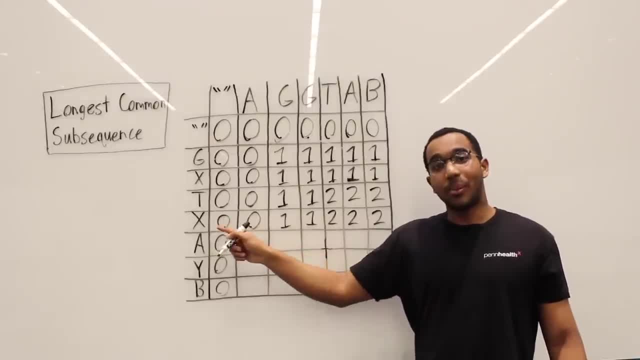 The answer to the subproblem with the A's removed is zero, Zero plus one. because I just removed the A, I just got a match and I can extend the longest common subsequence at the subproblem right here. So it becomes zero plus one is one. 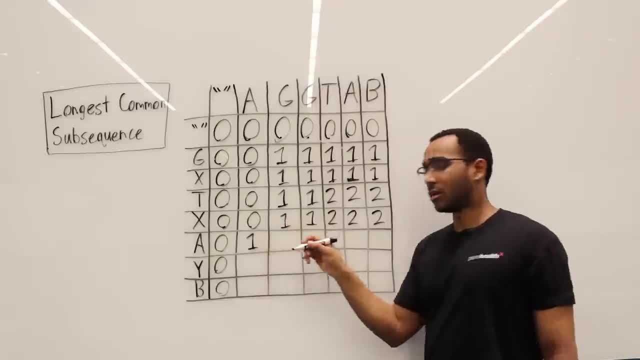 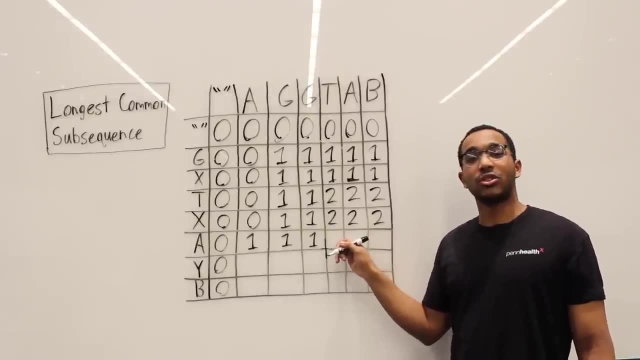 A and G mismatch The max of one and one is one. A and G mismatch The max of one and one is one. T and A mismatch The max of two and one is two. So A and A is a match. 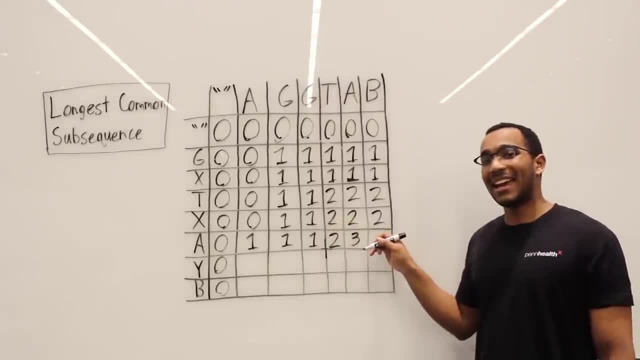 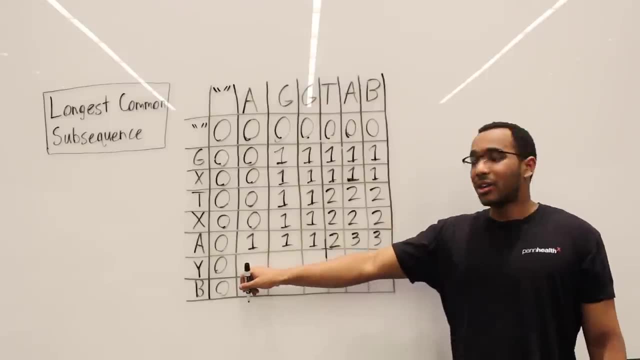 So what we do is two plus one is three, So B and A is a mismatch. So what we do is compete Three versus two. Three is the max, So why? So what we see here is: why does not match any of these guys? 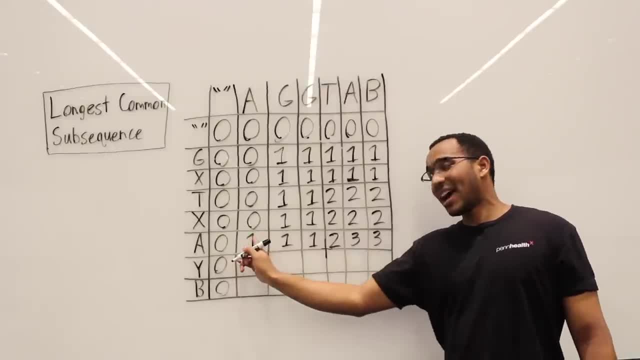 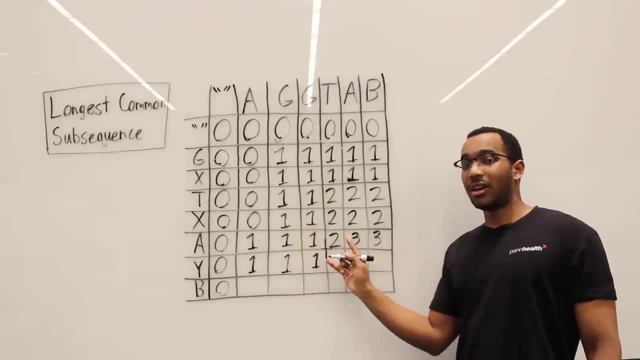 So why is just gonna have max operations happen? The max of zero and one is one. The max of one and one is one. The max of one and one is one. The max of two and one is going to be two. The max of two and three is three. 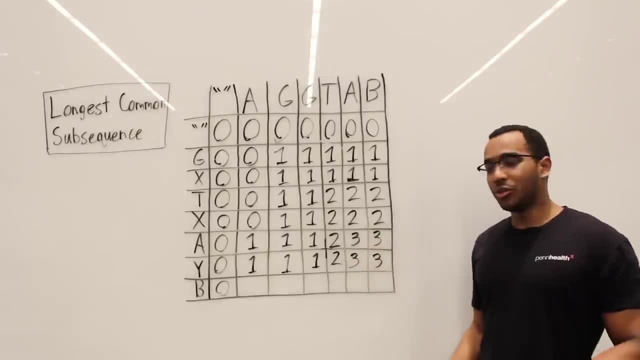 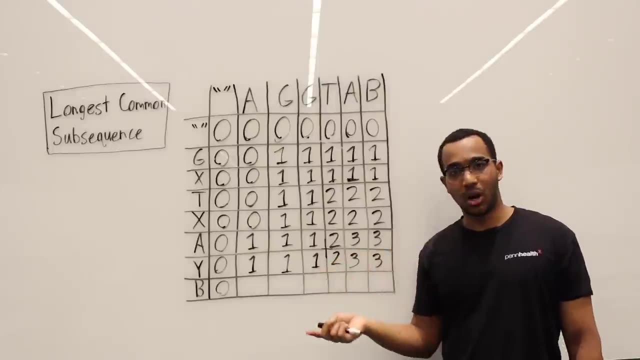 The max of three and three is three And why did I just rush through that and do these maxes? Why does not match any of them? So we would never do an operation where we do a plus one. We do not extend any longest. common subsequence subproblems. 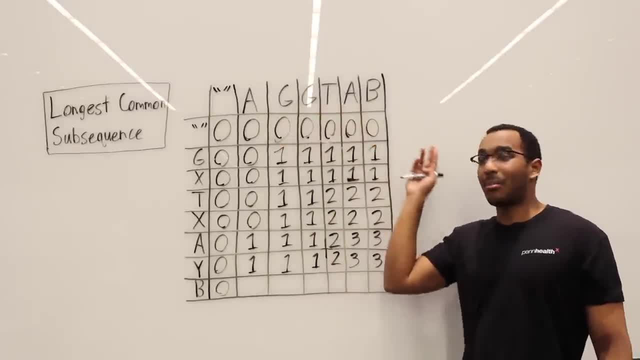 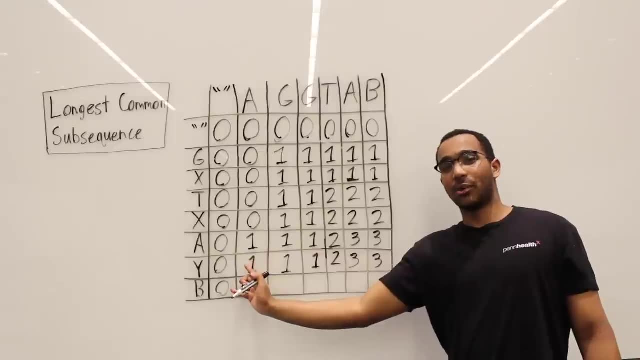 So what we are going to do is B, And we see that we do have a match B at the final position. So every position up to that, we are going to be doing max comparisons. So max of zero and one is one, Max of one and one is one. 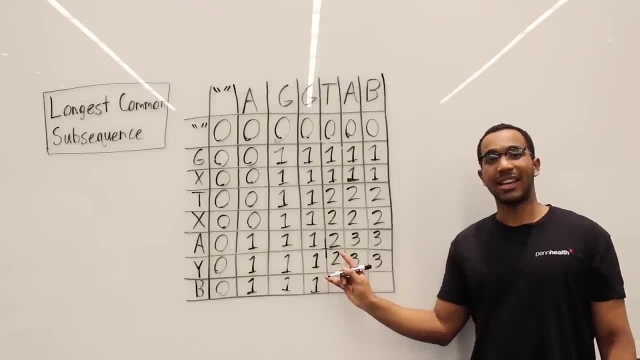 The max of one and one is one, The max of two and one is two, The max of three and two is three, And we see that the Bs match here Bs match. So what I do is I come over here And what I do is I do three plus one. 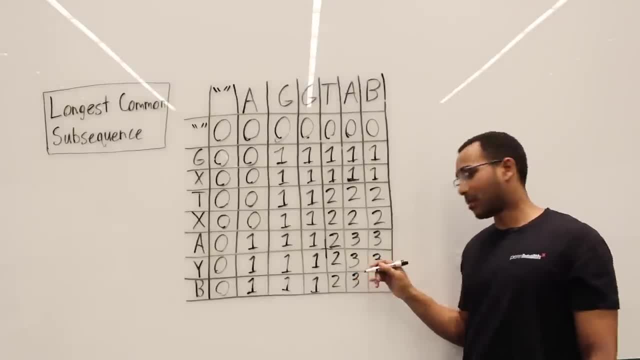 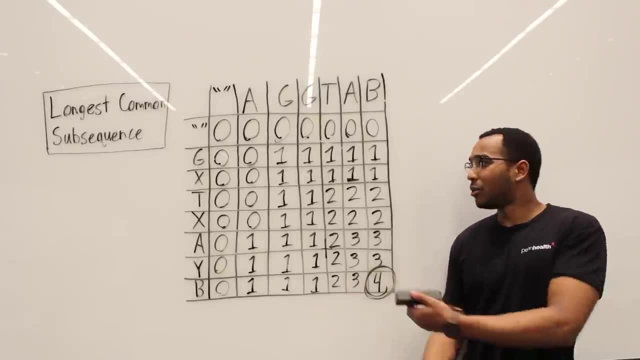 I remove both of the Bs, Three plus one, It becomes four, And the final answer for this problem is four. And is that true? Am I right? Am I wrong? I do not know whether I did this right, So let us see what these strings actually look like. 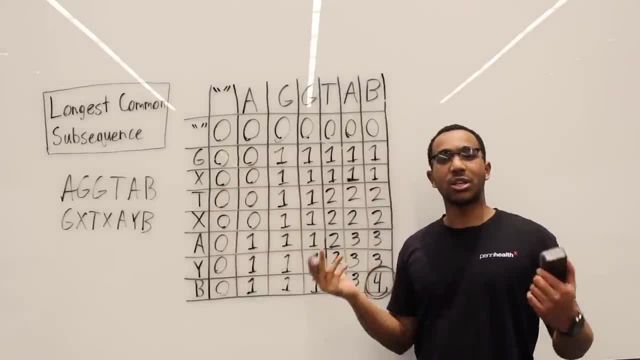 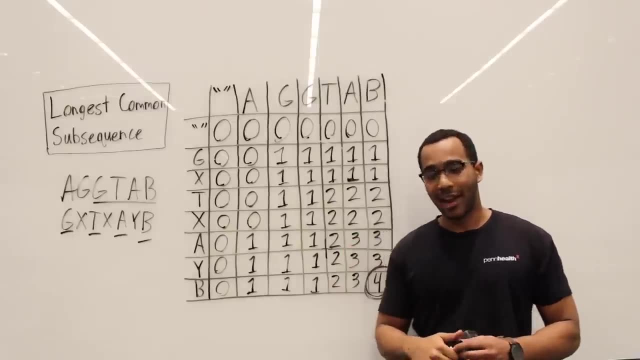 Okay, So do you see them? So what is the common subsequence between them? What is the longest common subsequence? And you see that our answer is correct. The answer of four is correct, And what we have here is the concrete answer of what this looks like. 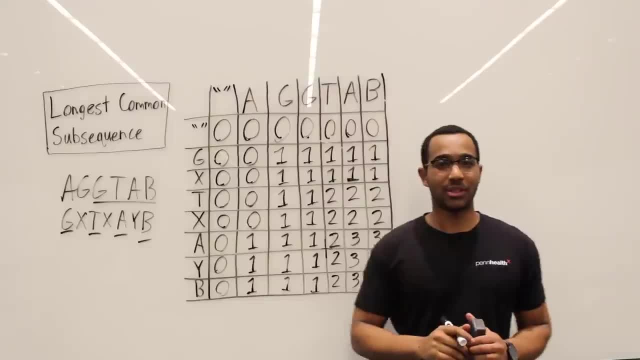 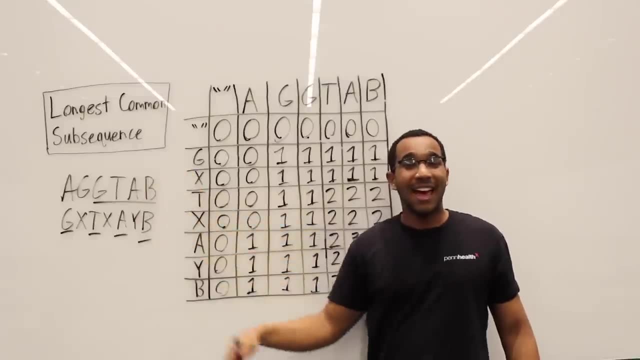 So here's our dynamic programming table. I don't want to make it about the table, I don't want to make it about memorizing this. I want to make it about understanding what is really happening. And okay, this is not intuitive at all. 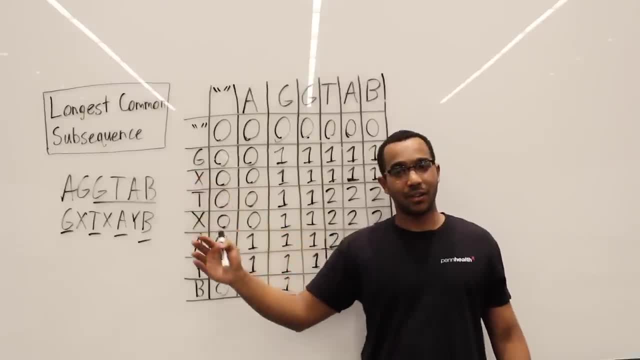 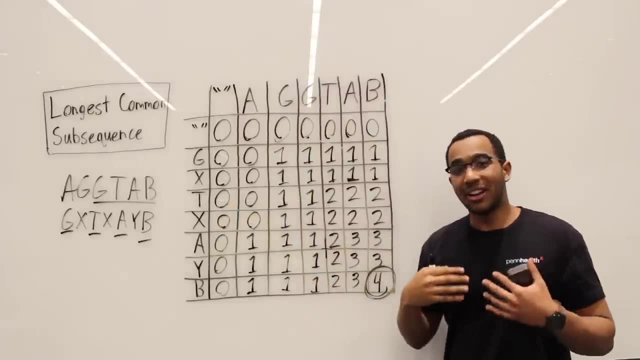 I'm going to be outright and honest. How are you going to get this in an interview? The thing is, the more you practice problems like this, if you know how to do the Levenstein distance, Then you're going to have a much easier time.